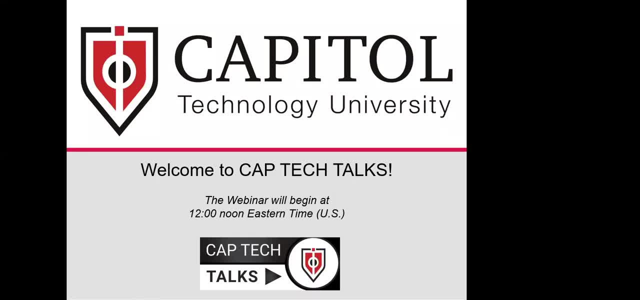 Hi, everyone. Bill here again. And we are just one minute out from starting. We're just about ready to begin. I'd like to welcome all of you who have just joined us. And if you've noted, if you have not activated your chat, please go ahead and do so. That is the way we'll be taking questions today. We do appreciate everything that our presenter is going to be doing for us today. So welcome. 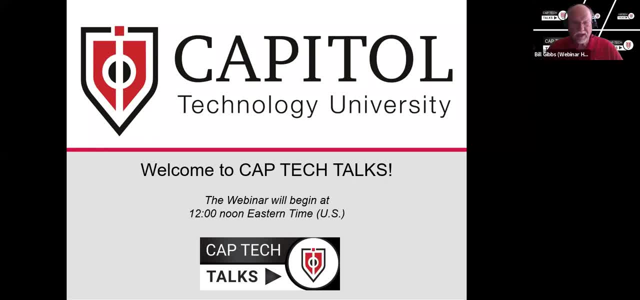 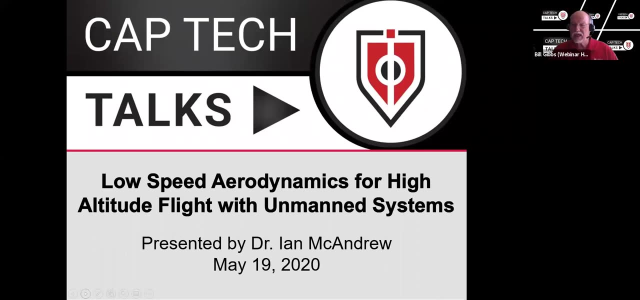 All right. This is Bill Gibbs and want to make sure that I can you can hear me. Okay. And we are ready to start. Welcome to the CAPTED Tech Talks, if I can say that, for May. And it is just a pleasure to have you here. Our presentation today is low speed aerodynamics for high altitude flight with unmanned systems, which will be presented by Dr. Ian McAndrew. 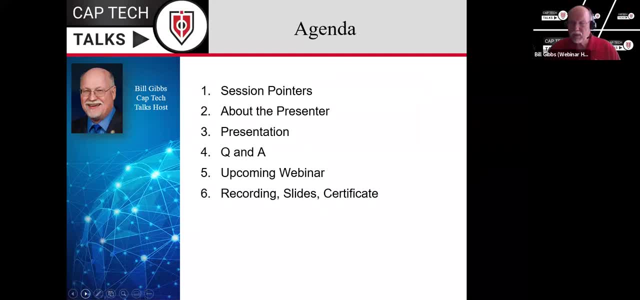 Here's the agenda that we'll be following today. We'll begin with just a few session pointers and then I will introduce the presenter, Dr. McAndrew, and then he will go through his presentation. We will be collecting questions as we go. And you can pose them at any time via the chat. We'll talk more about that. Well, after the Q&A toward the end of the presentation, we'll talk about the last webinar of the season, which is coming up in June. And also how to get a copy of the recording, the slides, and a certificate. 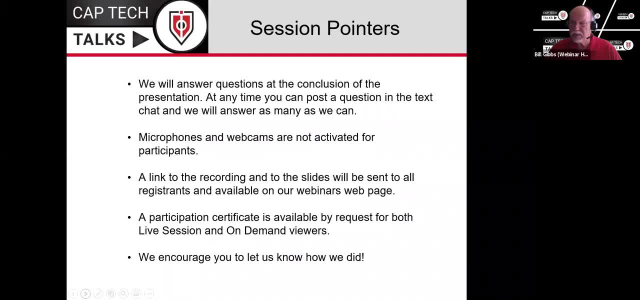 Of participation, we'll talk about all of those in a little bit. Here are some session pointers. We will be answering questions. Really, at the conclusion, but at any time you can post them if they happen to be germane to the discussion, right at the point. 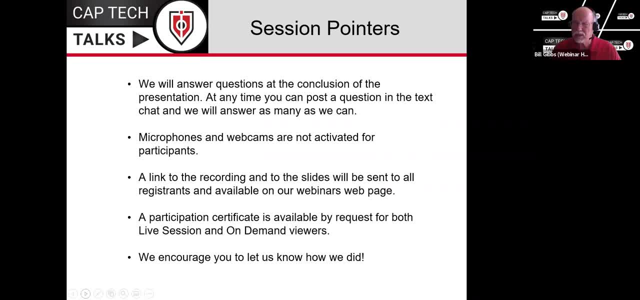 Maybe Dr. McAndrew, that will be at his discretion, will decide to take the question then. But most of the questions will be answered at the end of the presentations. 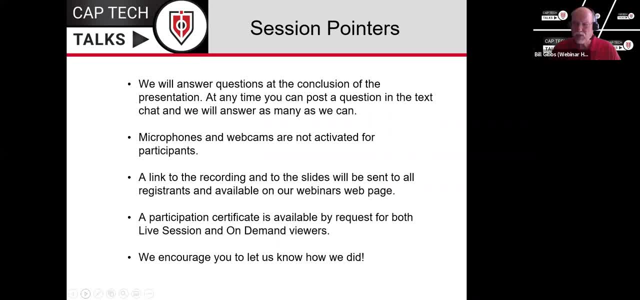 We're not activating microphones or webcams today for you. So if you do want to take a look. I'm going to leave you the question. I'm going to leave you the question. I'm going to leave you the question. to communicate with us please use the chat chat function we'll be sending a 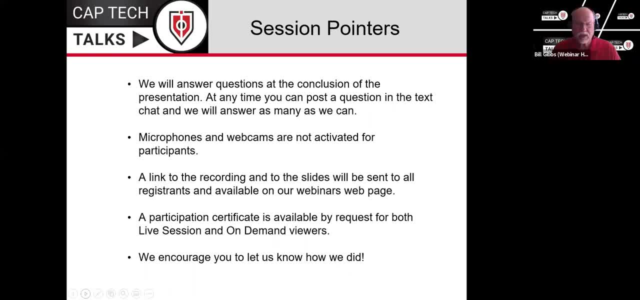 link to the recording and to the slides to every registrant whether you would join the live session or you're listening to the on-demand recording and that will also be available later in the week on our webinars web page we will offer a participation certificate that's available by request at the end of the presentation I'll talk about how to get that that's available to both live session those joining us right now and our on-demand viewers and we will always encourage you to let us know how we did you can do that via an email after the 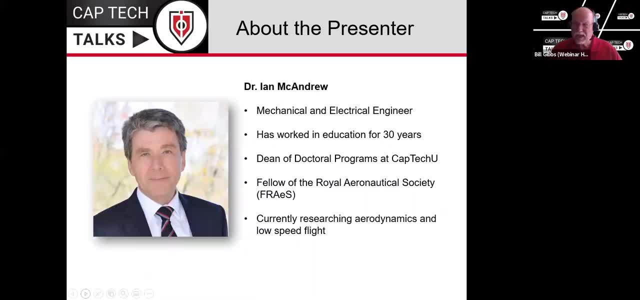 presentation is over now with that let me talk just a little bit about our presenter that is why you're here and I'm just really excited to have dr. 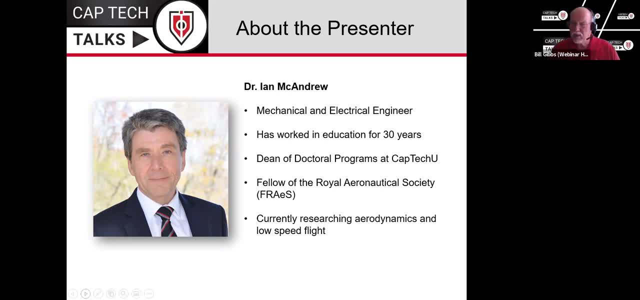 McAndrew I've had the chance to work with him quite a bit over the last few months our presenter is dr. Ian McAndrew you 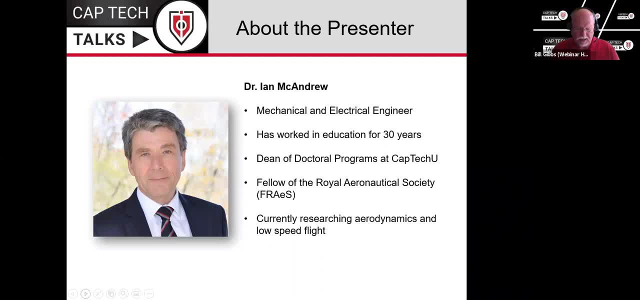 have a great time today and I'm really pleased to be here with you today professor Ian McAndrew PhD is a mechanical engineer who has worked in 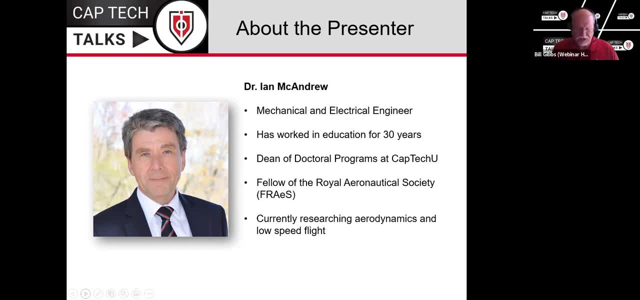 education nearly 20 years his teaching and research have been global starting in London and now with Capital Technology University where he is the dean of doctoral programs dr. McAndrew by the way is based in Europe but he has taught all over in 25 different countries he's published with many academics from all over the world and is a fellow of the Royal Aeronautical Society, the oldest professional aviation organization 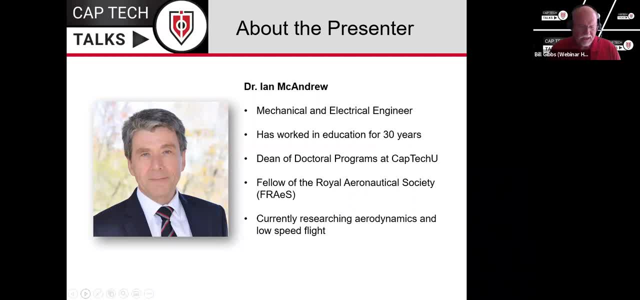 in the world. He has supervised over 80 PhDs and I suspect that it's many more than that now because that was updated last fall and he has over 60 peer-reviewed publications. His current research 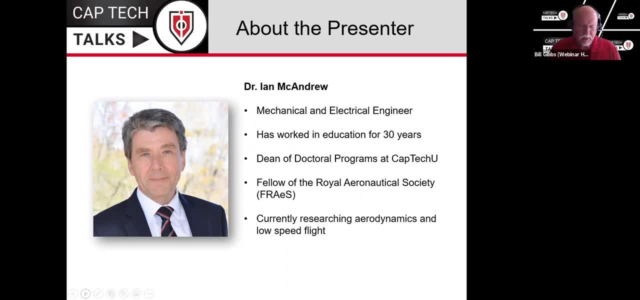 is in aerodynamics and low-speed flight. He's frequently invited to deliver keynote speeches and is the chair of several international conferences. Additionally, he's the editor or assistant editor-in-chief of several international academic journals. Dr. McAndrew will provide a bit more detail about his industry and research background during his presentation. Dr. Ian 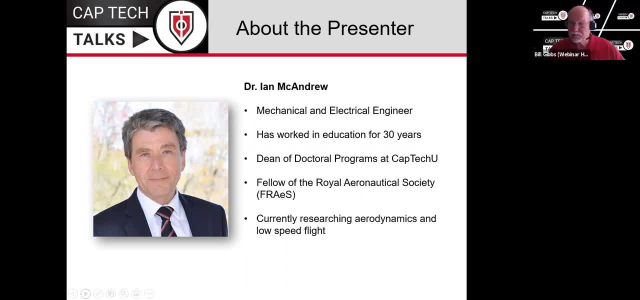 McAndrew, welcome. I give the slides to you. Thank you, Bill. Can you hear me clearly? I can, go ahead. 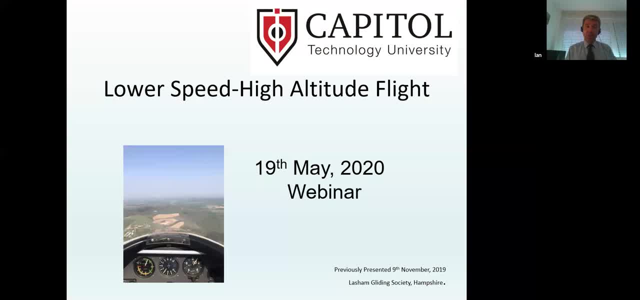 All right, well thank you and welcome everyone. It's nice to virtually have you here and to be able to talk to you. What I wanted to do today is to go over, as well as obviously the subject, low-speed, high-altitude flight, a little bit of background about myself and how my sort of logic and following this through into an area which, at the end, I hope you'll find is interesting and sort of reflect upon it for yourself. I've given this talk or variations of this talk and added to them over several years as it's been a sort of a slow burn project that I've been working on. 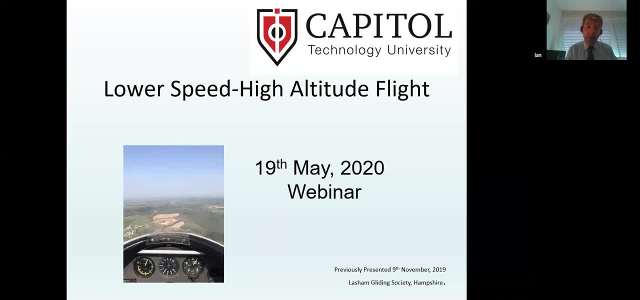 In comparison, I've been working on a lot of things that I've been working on, whether it's in person or in parallel with some other research to do with propeller design, 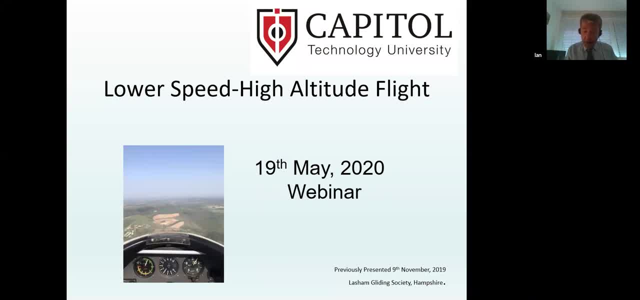 controls and different things like this. But I would like to start by quoting the great Stephen Hawking, who is no longer with us. And when he wrote his book, A Brief History of Time, which became a global success in the 90s onwards, he started out with the premise that he didn't want to put any or every time he'd put a mathematical formula in the book, it would half half the enthusiasm that he was going to put into the book. And that's what we're going to do today. 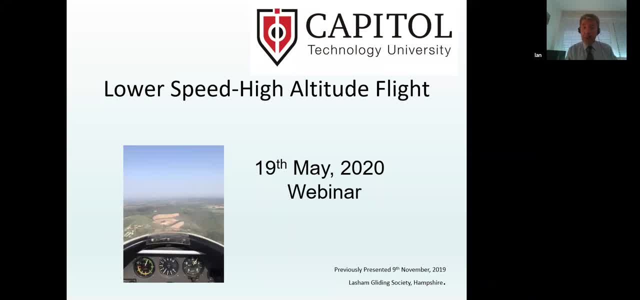 I'm not ignoring the math side of it. I'm just trying to talk about it and explain it, but also where my ideas came from and how I came up with this. Bill, can you advance the slide for me, please? 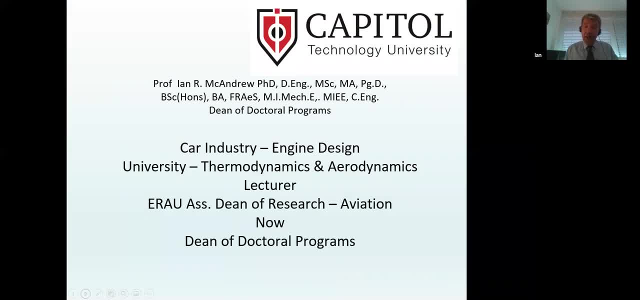 Okay. I never started out to be in the area that I am in now. I went to work in the car industry in the UK and was involved in engine design. And in particular, you know, an area which not a lot of people, it's a private thing I try not to share too much. My area of expertise was to design parts to break after warranty and did a lot of mathematical analysis and modelling of thermodynamics. After my doctorate, I moved into a university in the UK and was put in charge of the thermodynamics lab. Now, I had a sort of a professor that was more interested in his research than anyone else's. And in the thermodynamics lab was the aerodynamics lab. And the aerodynamics man retired and I was given because they ended in dynamics, running both of them. And ended up more and more in the aerodynamics side as a lecturer and getting involved with the research. I was then a professor at the University of London. And when I was then approached, I transferred from there to working with MB Riddle worldwide. And started as faculty, then ended up as a department chair. 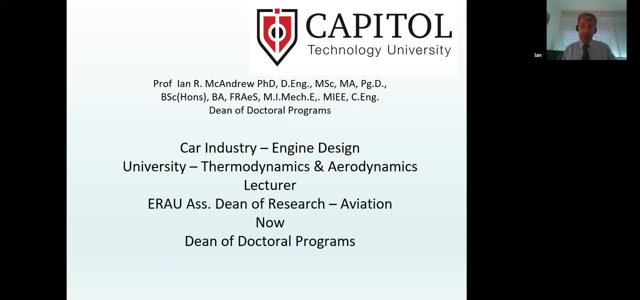 And as the associate dean of research on aviation, where I obviously spent a lot more time dealing with aerodynamics. Now, I've left there and I've come to work with Dr. Sims, our president, as the dean of doctoral programs. Now, aerodynamics is one sort of one of several sort of areas I'm very interested in. And we indeed have a lot of aerodynamics and we have a lot of aviation at the university now. But it wasn't a direct path to come in here. And I had a very convoluted way of looking at different areas and different things. And ended up is where I am with a sort of a mismatch of different approaches. If you could advance the slide please, Bill. 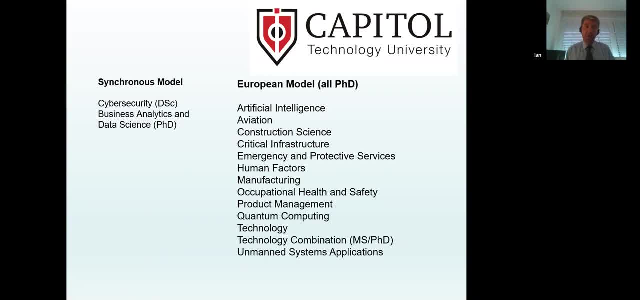 Now where we are now. And several of you I've noticed, actually students at the university and I run the synchronous and non-synchronous European model PhDs. Traditionally Capital on the left has been a leader and successful leader in cybersecurity and business analytics and data science but over the last few years we've added these programs on the right hand side and you can see aviation and human factors and even manufacturing we have aviation experts in the manufacturing PhD are looking at areas but you can't look at areas on its individuality now. Areas all come together and we need to be 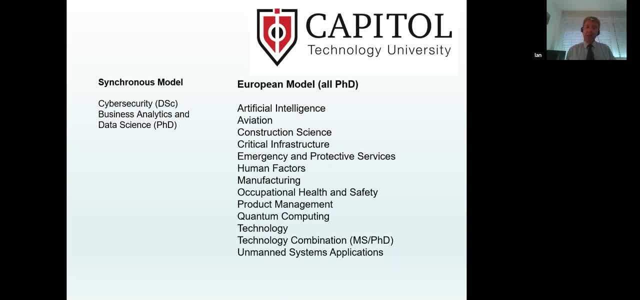 thinking about how they work. If we go back years ago we can talk about you know someone designed a car, someone designed an aircraft, someone designed a bridge. That no longer happens, we work in systems and we work in terms of dealing with lots of different areas and what I choose to do is I'm going to talk a little bit more about what I do in the future. So what I'm going to charge you today with and hopefully that you'll come away is to think about not just your own area but where it fits in with the other areas. There are areas where probably your obvious knowledge is not obvious to everyone else and vice versa and this if we look at it I think can give us a chance to look at research and expand research and make it more useful and relevant. Next slide please Bill. 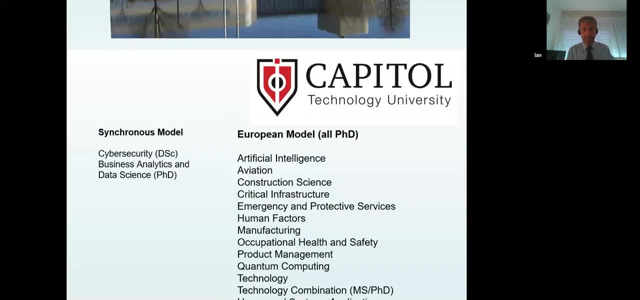 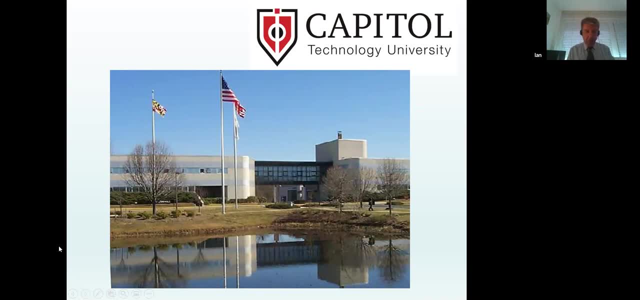 Now anyone that's been on campus will recognize this photograph here. This is the main entrance to Capital Technology and we look at the building, the ponds looking lovely, the sky is blue and everything. Let's think about the history let's think about Capital Technology. We've been evolved from communications with the Navy and we've evolved and expanded to become college and our university. But let's think about where we are and sometimes we walk around and we don't always see I think what is there. We miss opportunities. Now look at this building and the next time you're on campus the entrances to those two sides of the building have a very large radius on them. There is a glass corridor that goes from one side to the other it's elevated. This was designed from the influence of architects in the Cold War where if there was going to be a strike or a sharp corner or a sharp corner is bad a radius on the corner of the building deflects the explosion. The idea of the glass bridge between them that is the sacrificial part that if one part of the building gets hit the other doesn't really get damaged because that part collapses. Now what does this got to do with aviation? Well next line please 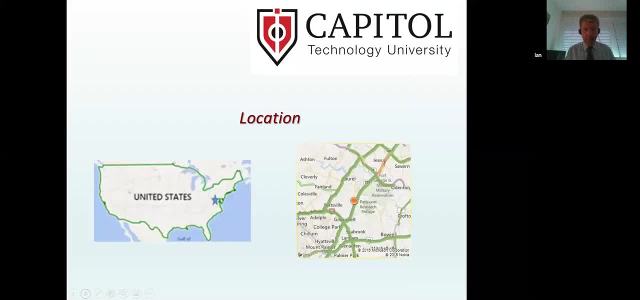 Bill. If you didn't know this is where we are the star on the map and if you look on and you can see where we are based around but for those of you are very local you know that around us there are a lot of DOD and three-letter acronym agencies where we actually educate students and they go and work there we have people have been working there and retired and come to join us and teach we have adjuncts that are around we're in an area which in the previous history was a target for people and our building was right in the middle of what you would call a wonderful target area and we're left with those legacies and sometimes we design things and we forget why 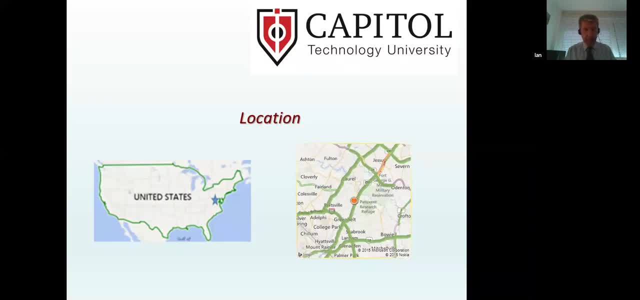 they're designed and we totally don't understand what it was there and we assume that everything that was completed in the past is successful was correct and is relevant today next slide please 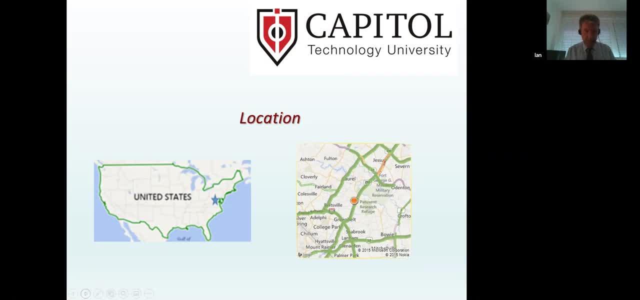 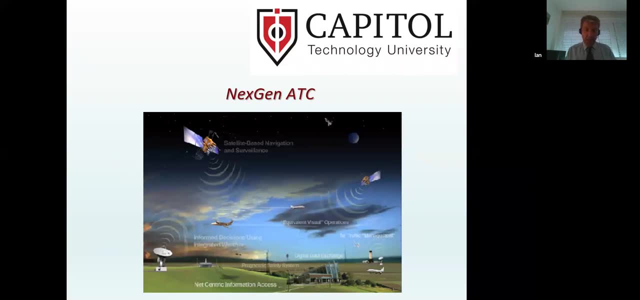 now what is happening aviation in many ways there are a lot of excitements at the moment there may be a lot of sort of a depression in terms of look the 737 max hasn't been sorted out we can't fly many places it could indeed be the end of the boeing 747 as airlines actually put it out to grass because it's not needed and there's less command and all these things that we have but we have this thing called next generation which is a true satellite global link of all aviation around 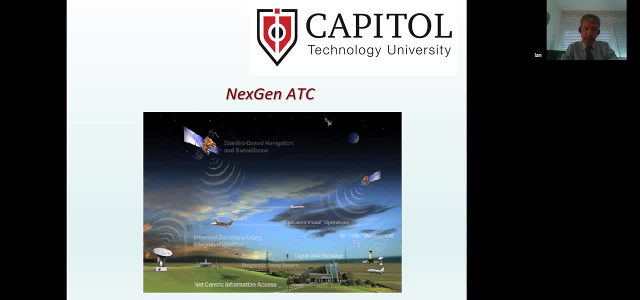 the world we're talking about integrating aircraft that can take off and land we can work out the optimum landing patterns that if we're trying to land a jfk on a saturday night or friday evening or we're trying to take off from jfk and we're in a queue and the pilot says we're we are now number 27 on the list for takeoff to remove these bottlenecks and this is an important thing that's going to happen and it's starting to happen and it's rolling out now there are reasons for that because in aviation pilot error air traffic control error have all caused concerns and people are worried about them but we are now in a situation where we can have uavs potentially flying with commercial aircraft we can have the amazon dream of all these drones flying around delivering our parcels and packages that we've ordered but there's still a big barrier to cross and it's not necessarily technology it's sometimes the human perception do we want to be landing when a uav is flying near us what happens if a uav accidentally went into an engine of an aircraft taking off or landing the thought isn't worth considering because it would be horrible and one crash caused by a uav potentially could hold back that particular industry for years we saw a slight delay in space exploration after the horrible disaster of the first space shuttle explosion 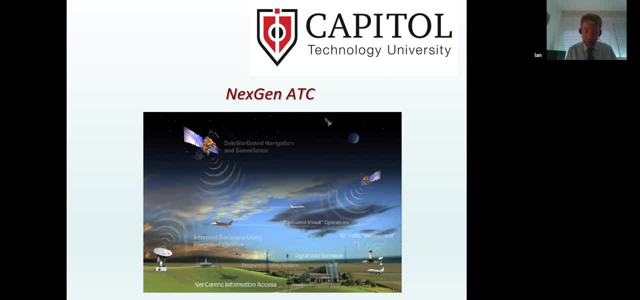 in aviation when we fly millions that has a bigger connotation and it's important when we move forward we move forward and we make the right decisions and we think about sensible solutions and i would like to quote a particular thing and some of you may be familiar with the film jurassic park and there was dr ian malcolm and they'd seen all the dinosaurs and they came to have this meal and they're all excited and they're talking about everything and the mathematician or the mathematician dealing with chaos theory was very uninfluenced and they said what's wrong 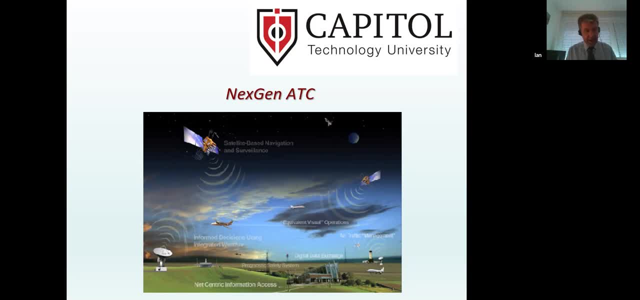 and he said you stand on the shoulders of giants in scientists you've made these dinosaurs dinosaurs had their chance they didn't survive and they're gone 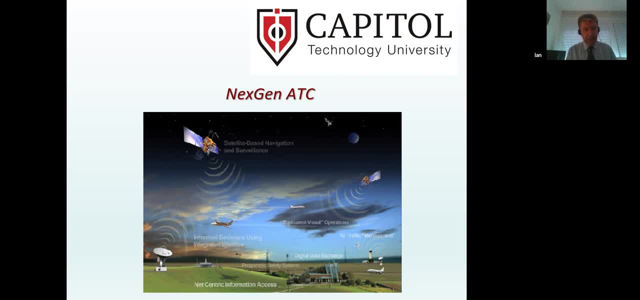 and you missed what is very very important in research and science and technology and that is you didn't ask should we do this when you ask the question can we do it now next generation if we ask the question should we be doing it should we be flying drones in the same commercial airspace as we would fly on our holiday or business trips now i'm not trying to try to answer that today but i would think about it you know if we can separate them that is good but if we don't separate them we can't use them so advanced as we want to now next slide please 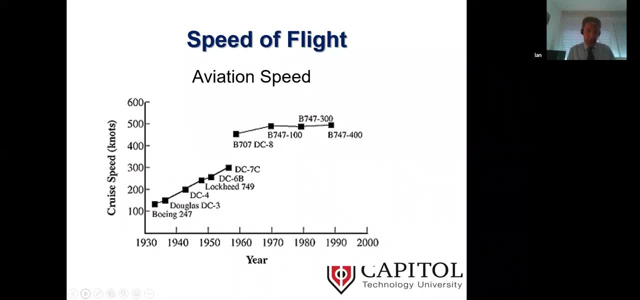 a little bit of a history lesson here if we look from the early planes of boeing's 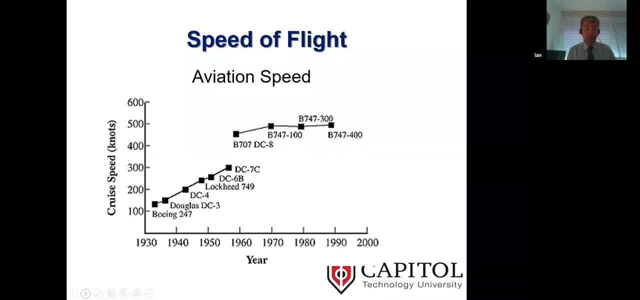 seven four two four seven the douglas dc3 and all these planes we ended up with the dc7c which was the most at its time advanced propeller plane in the world very very advanced with this design of propeller blade variable pitch and many things like this but it had a maximum speed of around about 300 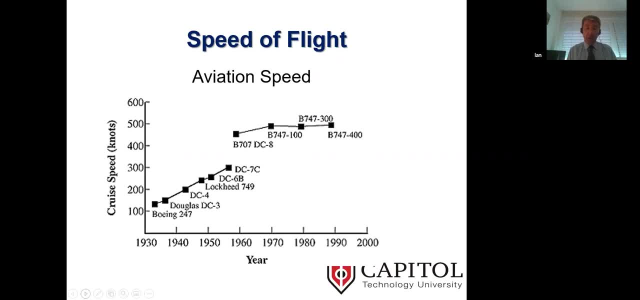 we can see there was a big jump between the 50s and the 60s where much faster speeds were possible we jumped from about 300 to the upper 500s and quickly to the 500s approaching the speed of sound now that difference between those two we all know is the jet engine and we know that that's the reason why and it's a legacy a fortunate legacy from the second world war where money was invested and the jet engine was pushed forward 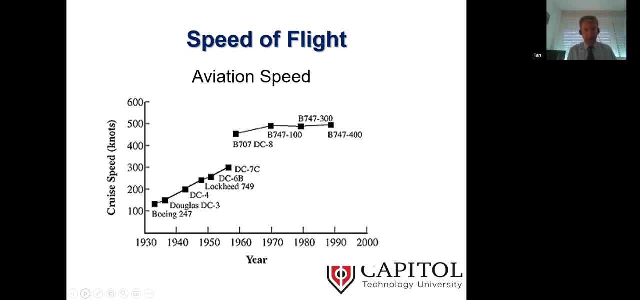 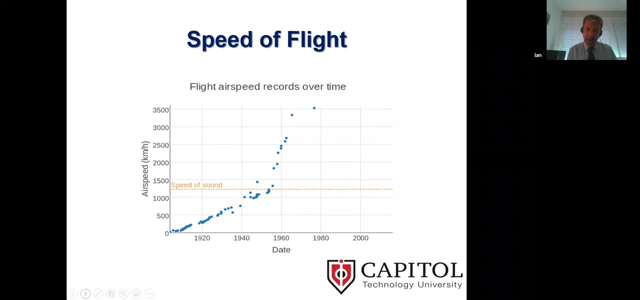 and we can fly across the atlantic or the pacific in times which are reasonable as compared to the old cut planes with propellers now next slide please now that's increased and we broke the speed of sound chuck jaeger took us there and if we look at the speed of sound and we look above it and the different aircraft these are all military aircraft all of them except one and i'll talk about that in a minute and we now have planes flying at three and a half thousand mac4 mac5 we're having research done on hypersonic planes now where we can go above mac5 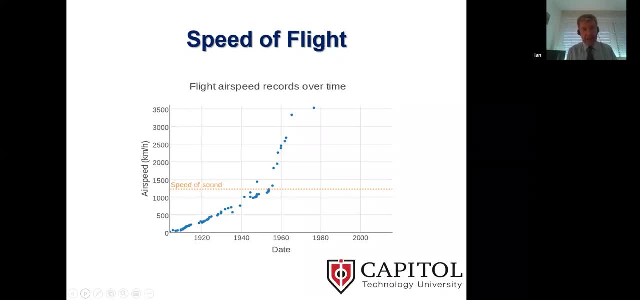 even to mac 10 and get to australia in seven hours several hours but is that what we're 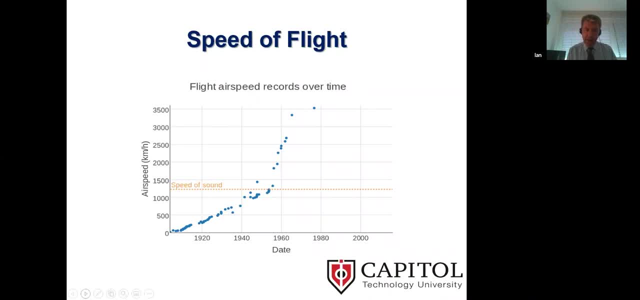 thinking about and is that really where we're going and trying to integrate high flight and uavs next slide please 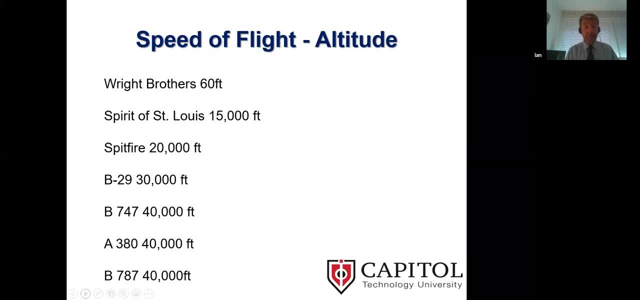 again it's not just the speed let's think about the altitude the wright brothers about 60 feet that wonderful breakthrough in science the spirit of smith 15 000 feet and the spitfire and the p1 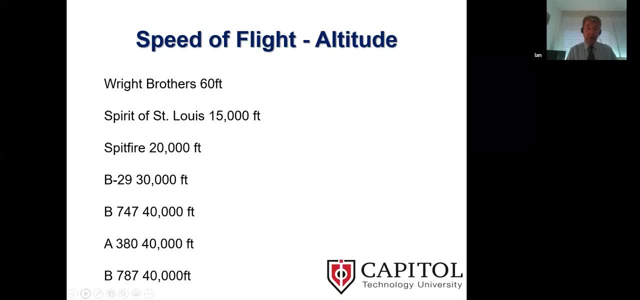 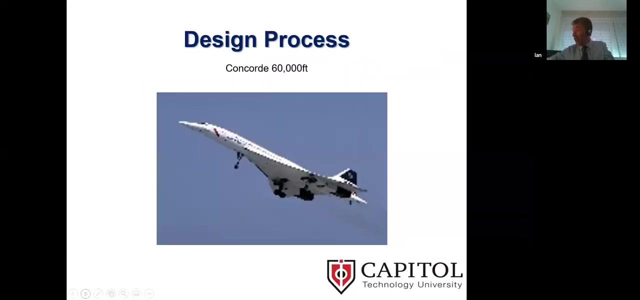 mustang and p51 mustang 20 000 feet and then came along the b29 with its pressurized cabin which took it up to 30 000 feet where people didn't have to be cold with big leather jackets on to be flying and then look what's happened the 747 the 380 the 787, there's a service ceiling of about 40,000 feet. You know, you might be on an aircraft that flies at 42,000 feet, but that's probably the altitude that you stay at. Next slide please. Again, let's think of this Concorde. Now in my 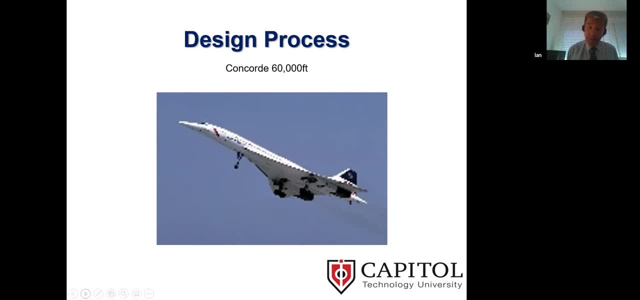 opinion, an amazing aircraft. I was fortunate enough to fly it, but leaving that aside, it had a service ceiling of about 60,000 feet. In its day, it had a speed and altitude that was equal with many military aircraft. And I cannot think of another example, and if you can please put it in the chat, where after we 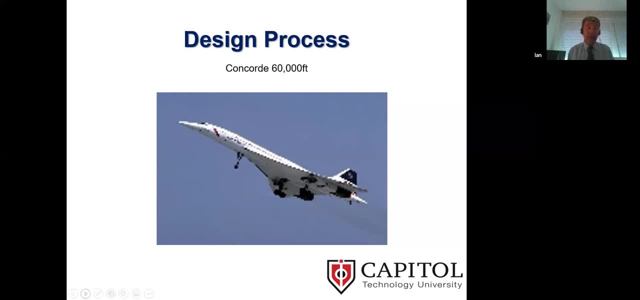 stopped commercial supersonic flight, where we've ever taken a technological step backwards? Because we have. You cannot fly supersonic commercially now. 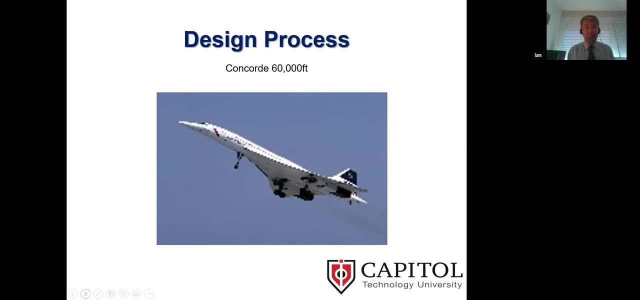 It has to be in a military jet. Now between 60,000 feet and 40,000 feet, there are mainly military aircraft. They're not 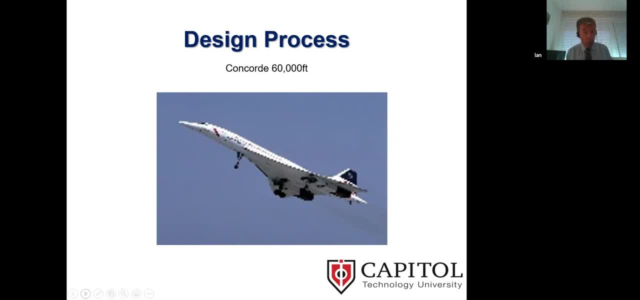 everywhere. There are parts of the world at the moment, perhaps there's more than normal, but there's a whole area between 40 and 60 thousand feet which you can fly, but hardly anyone uses it. And this is my idea. Why are we not using UAVs at this altitude? Now when I started brainstorming this a little while ago, you come up with the standard offers and the standard problems and different things. 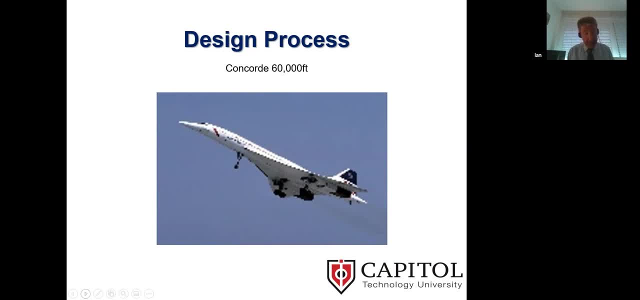 but this is where I'd like to introduce and talk about the problems and where we miss from the past and we've forgotten some of the past to look at the future. 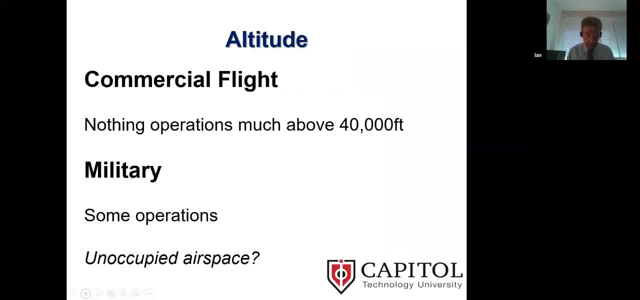 Next slide please. So again, military, we can keep away from military UAVs. 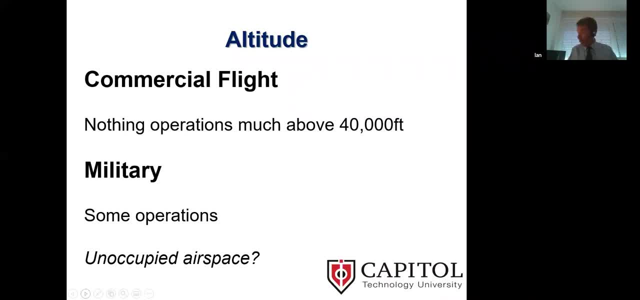 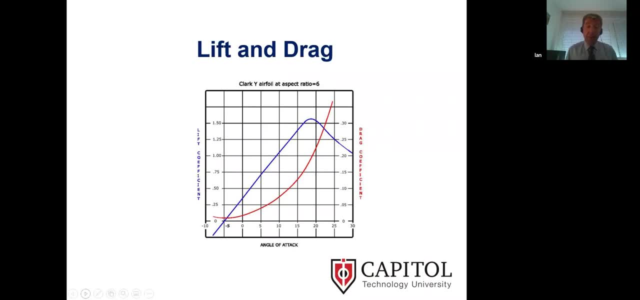 Commercial, why not fly above it? Next slide please. Again, I'll try not to bore you too much but we need to go over some of the basic things that we're talking 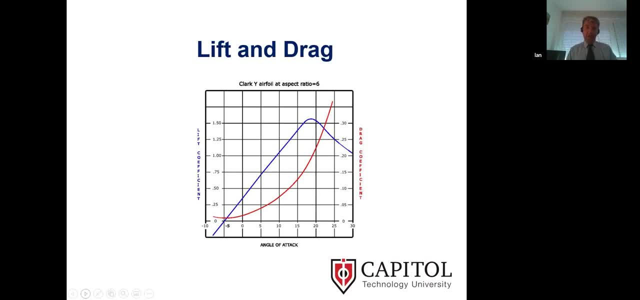 about on the problems. Now this is a graph of lift and drag, and I'm sure many of you here understand it, some of you may understand it but just give me a couple of minutes to go over some of the basics. What this is showing for a particular design and configuration of an aircraft. We can increase the lift by doing a variety of things, with the flaps and slats of an aircraft, or even twisting the wing upwards. Along the x-axis you can see this is what we call the angular axis. The angular axis is a particular area of the aircraft that is of attack and I'll come back to that in a slide or two what we have is the red line as we look at ways to make the drag as we look at ways to make the lift higher as we've everything we increase the drag and there comes a point and 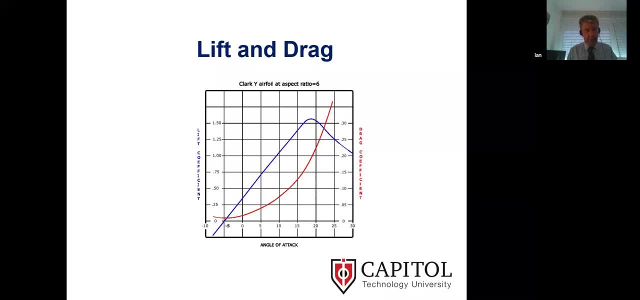 that on this graph really is where the red line crosses the blue line that's where planes fall out of the sky now we know this and there is an enormous amount of research and if you're into this area or not you can go and buy books and you can download information that will give you the profile cross section of any wing and will give you many of its characteristics for lift and drag how you would design this angle of attack how would you would use it and everything else now this is very advantageous when we're coming to land or take off the next time you look at the back of a jumbo jet there are three little mini wings that come out three slats that come out at the back to increase the wing to give it more lift to change that angle of attack and it increases the drag significantly but at low speed it's not so much of a problem next line please 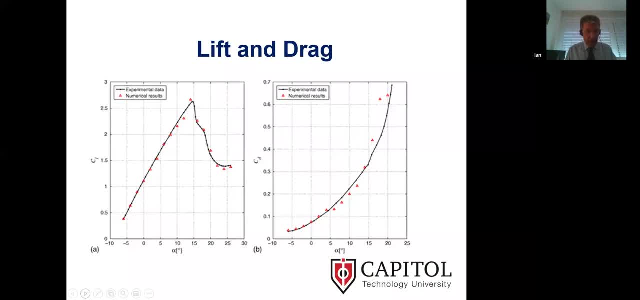 now here's a some modeling that we've been doing and I introduced this here because when I was looking at this I thought this is interesting now you look 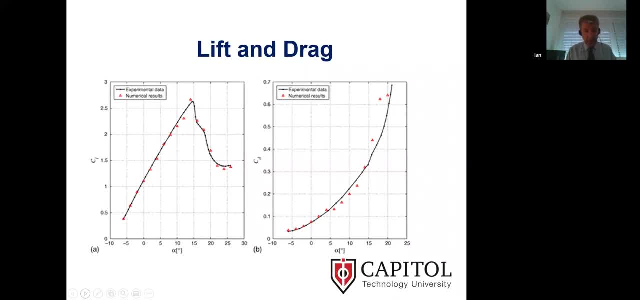 at the lines that we have and these are the lines that we have and these are actual real data for lift and drag it's not as smooth as you would see in a normal plane but if you look at it and look at it carefully it's the angle of attack and the lift and the drag and again the next line please Bill there's nothing in that lower end there nothing at all they haven't bothered no one bothers to look at a negative angle of attack below 5 degrees people haven't wondered why should we be doing this? doing that and I started thinking about this and you think well I can see the reasons why I can't understand why you know because you don't want to fly plain with a lot of drag because it's very expensive in the fuel the only time if you're a commercial pilot and you want to increase the drag is maybe if you're burning off fuel because you have to do a landing and there's a problem but no one's looking there and I'm thinking to myself oh I wonder why you know what made them stop and then I'm thinking about lift and drag again and then I'm thinking about lift and drag again. 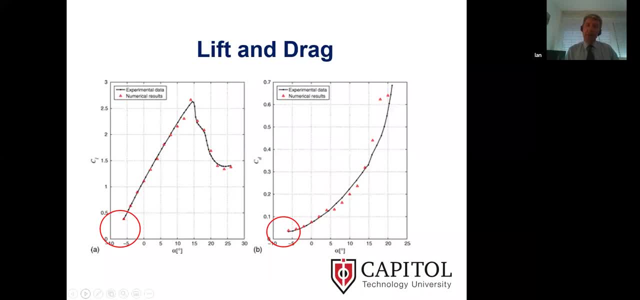 and I'm thinking about takeoff speed and then let's go if you think about the actual Wright brothers and the Spirit St. Louis then the Spitfire and all the other planes that have come along it didn't take very long and probably only about ten years before the speed of an aircraft was getting substantial they were getting bigger more complicated twin engines and different things like 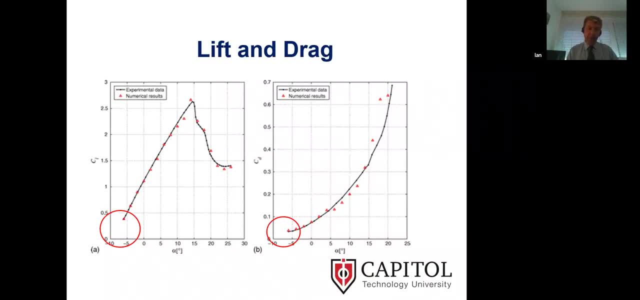 this people ignored the speed and when you look at areas for the coefficient of lift then you start calculating them they have coefficients in them and this made me start thinking again and the next slide please 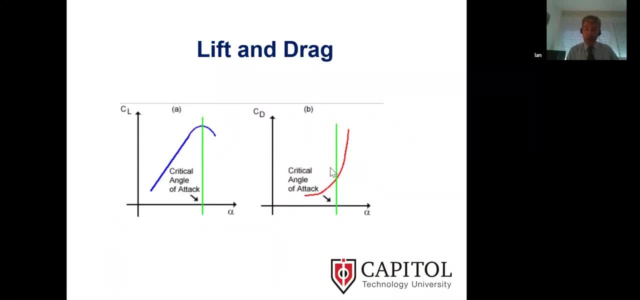 now again remember on the previous ones I've been trying to show what we talk about in terms of nice smooth curves I've added to this and this is called the critical angle of attack and again I'll clarify this in in a slide or two this is a very important thing if you go above that critical angle attack if you were ever been in the cockpit you will hear a certain noise which pilots don't like to hear and that is a warning sound that you're approaching the stall the stall means that the weight of the aircraft is very very close to the lift 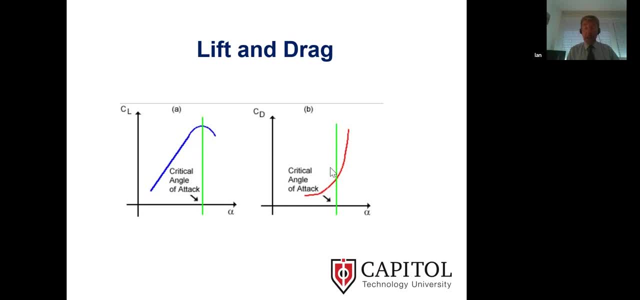 of the aircraft and it's very dangerous particularly on landing and taking off and even more so when you have different situations and different lightings and where you have ice on various parts of the wing it changes all of this and if you're ever in an airport and they say we have to de-ice the plane or something like that don't think it's 20 minutes 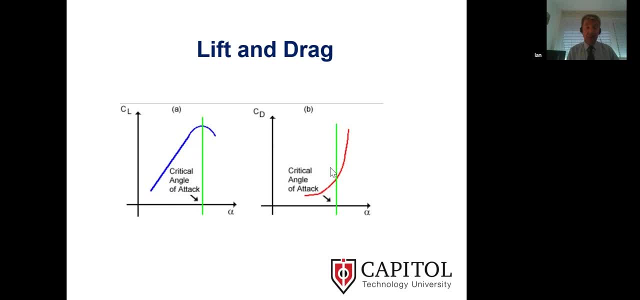 delay think this stops me dying from taking off so it's important to do these things now the next slide please 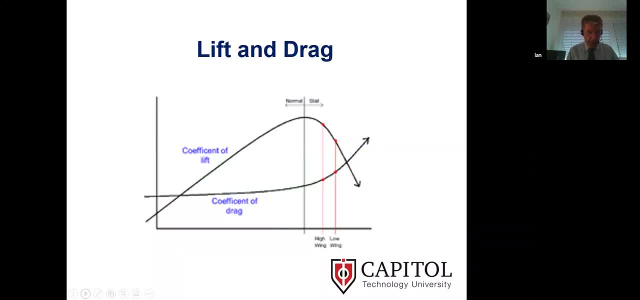 again and it's interesting if you look at some of the graphs without going in very deeply if you look at the coefficient of lift you see nowadays it never goes to the zero zero point there's always a positive form of lift but what these diagrams and what the charts and the data and the information do not tell us is the values that happen at incredibly low speed we don't 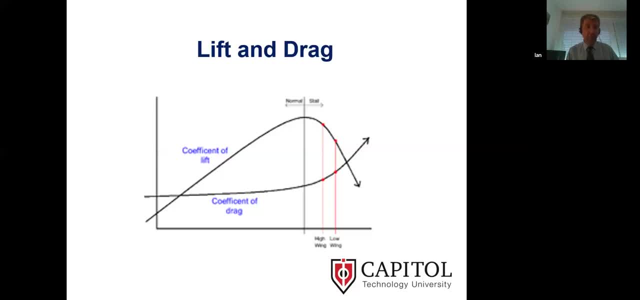 have any aerodynamic data that is generally available or even bothered to be researched which is very low speed and extreme levels of angle of attack on a plane because almost every single aircraft doesn't want that so why measure it why spend all that time 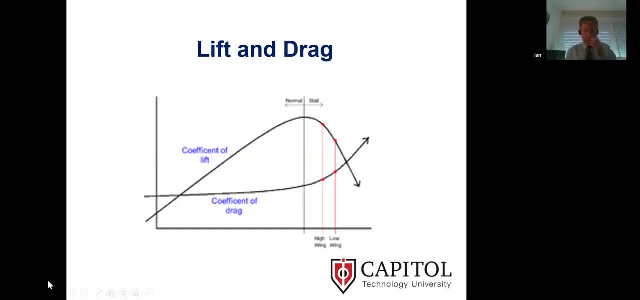 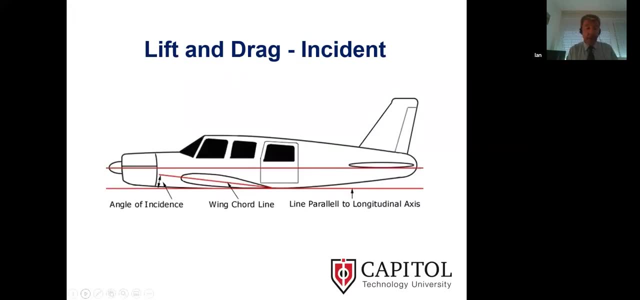 collecting it now next slide please very simple plane here the red line in the middle at the top 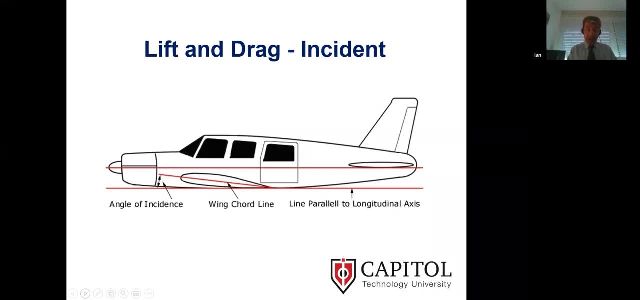 is what we'd call the center line and if you look at the cross section of the wing there we use this 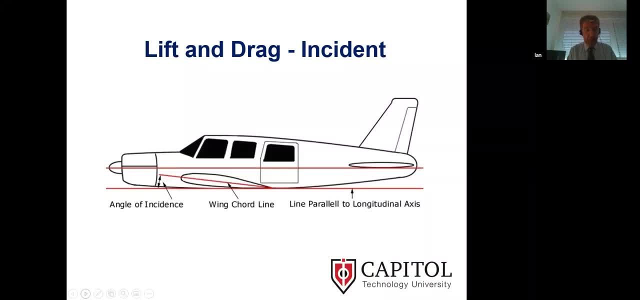 phrase called the cauldron and that's the point from the nose to the tip at the end now one of the things that we're going to do is we're going to do a little bit of a twist on the wing where it hits the aircraft not a lot but we put a little bit and at the end of the wing there is probably no twist 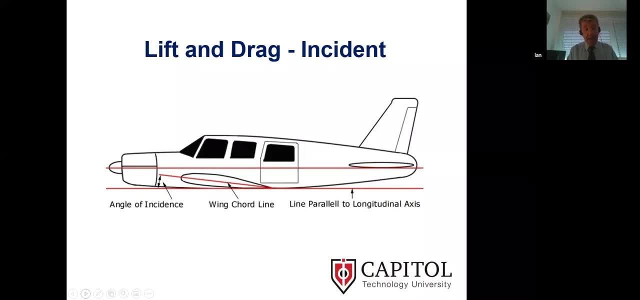 or no angle of incident the reason we do that is because the higher the angle of incident that is where stalls start if we detect the storm area and then the control surfaces the little bits that move at the end of the wings at the back 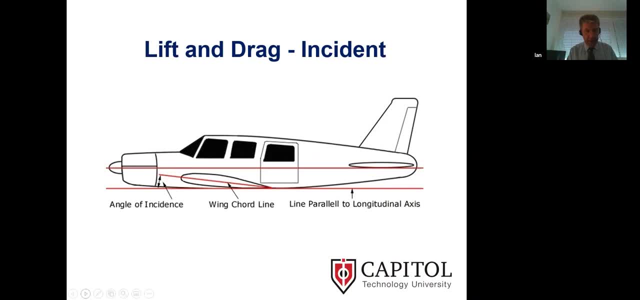 they're not affected by that storm or where the air doesn't flow smoothly and you can control the plane and get it out of the store so there's no need to have big angles of incident or anything 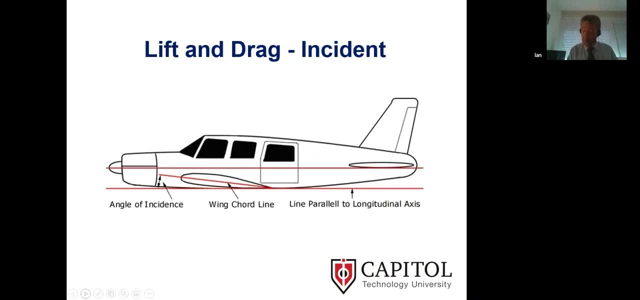 else like that but again this got me thinking and if you look on the next plane next slide please 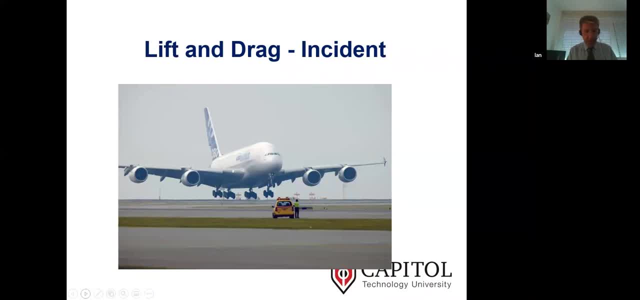 now here i think this is a wonderful plane i've flown on the top and i've flown on the bottom seats and various on the 380 an amazing plane i like to think i know a lot about aerodynamics but when i look at this plane taxing along a runway getting ready to take 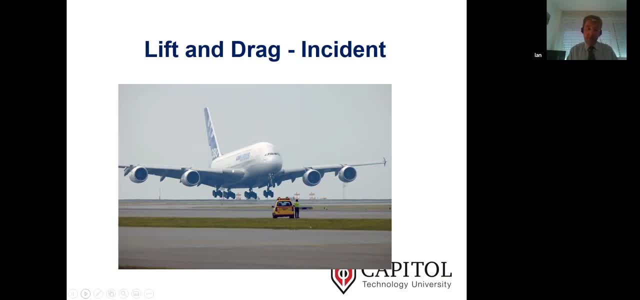 off i still look at it and think it's not going to take off the runway is too big it's too heavy surely it can't fly and it seems to go along at a very slow speed 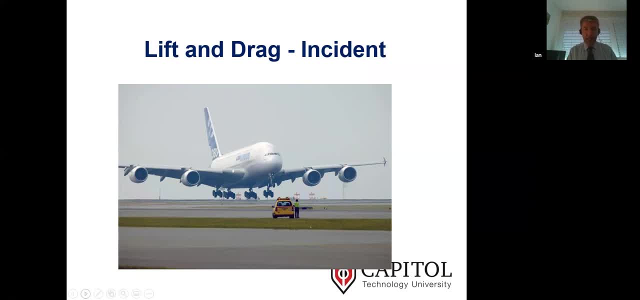 and then it takes off in other words the pressure under the wing is greater than 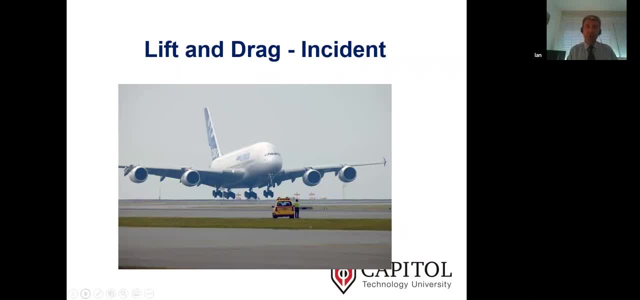 the pressure on the top we get a form of moving forward buoyancy as i call it and then we take off if you ever see this plane look at that angle of instant it is absolutely huge it generates an enormous amount of lift but the downside is it creates a lot of drag in level flight hence the four very powerful engines which like to drink gasoline or aviation fuel at a very fast rate next slide please 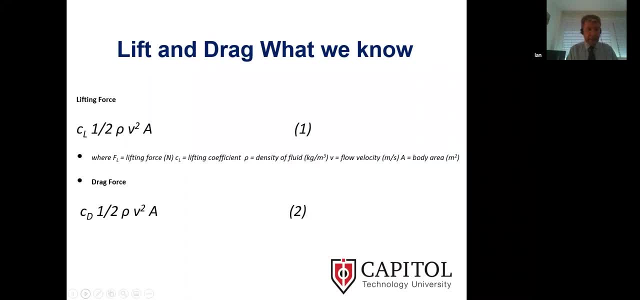 now here's the bit where hopefully some of you won't be too bored i kept out all the rubbish and i've tried to ignore some of the things and just put down the bare minimum 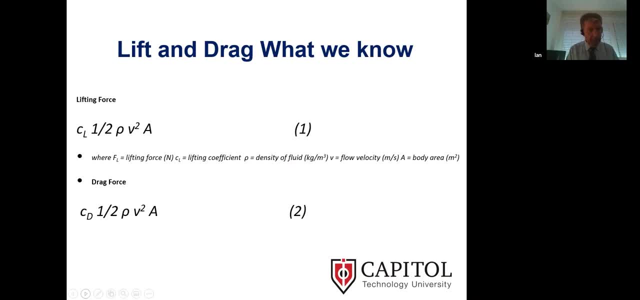 but what we do for any aircraft wing we calculate something called the coefficient of lift and if you look on formula one the coefficient or the actual force that lifts the plane up we multiply this coefficient of lift which is an approximation but a reasonable one of half rho v squared and if you remember any of your physics classes that's the kinetic energy of air where rho is the density of air and rho is the density of air and rho is the density of air and 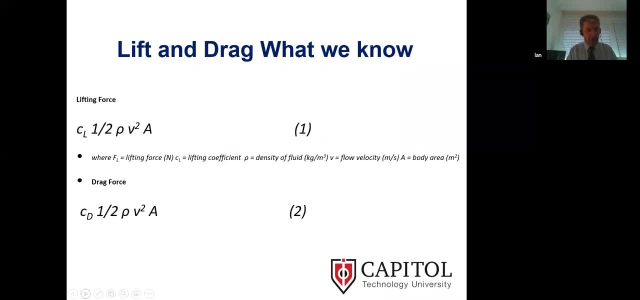 v is the velocity squared and a is the cross section of the wing 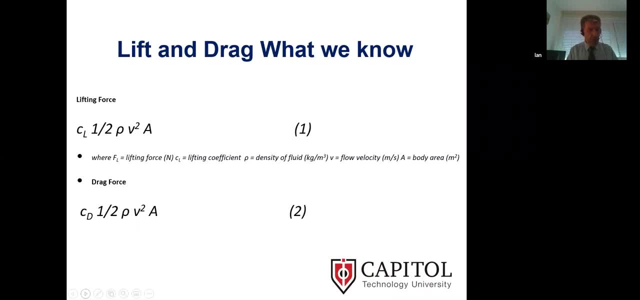 now the cl is pretty good for straight and level flight it's an okay estimation for takeoff and to give ourselves that extra lift that a we increase on an airplane by the slats and the 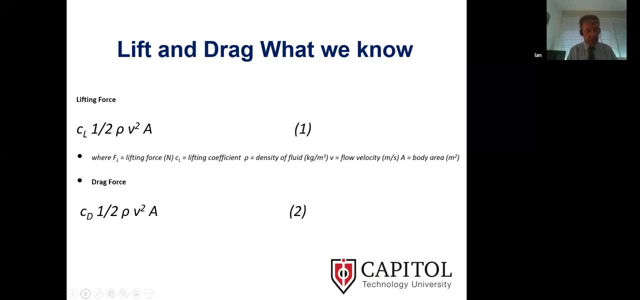 at the back and the slots and different things and if you look on a plane next time you take off how the wind gets bigger before it takes off and everything else that's to give you more lift to take off 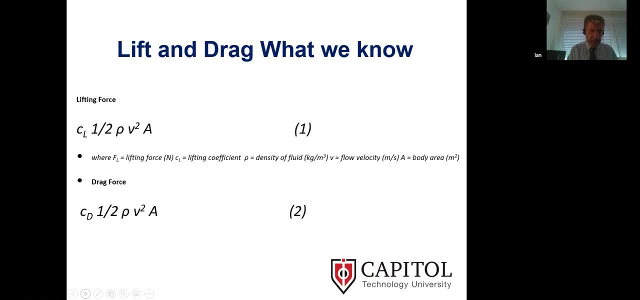 but also we calculate the coefficient of drag which is very similar it's the same formula except as the drag is of the coefficient of lift there we can work out these values and i'm thinking to myself you know we just don't know about the coefficient lift at certain areas we don't know about the velocity at certain levels and how that influences and this is where again i think i've reached the critical mass there and started thinking about the physics the next line 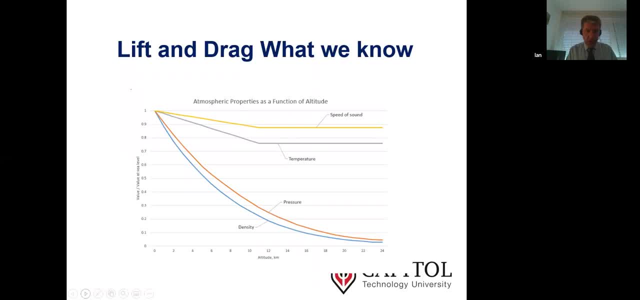 Now this is a graph that i dropped and it's an unusual graph you might not have seen anything like this before but it's one of my brain stormy things and on the left hand side we have one at the top now this is the value the standard value at atmospheric level at 20 degrees celsius 68 degrees Fahrenheit on a normal day with normal atmospheric pressure and what i've plotted along the bottom is the altitude as we go up now watch as we go back and shell is very high and now what we've calculated along theезжarsethis long üçe 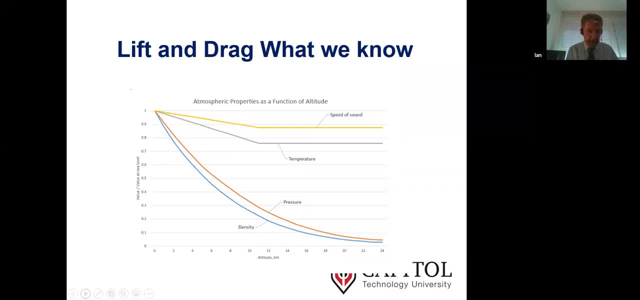 do we know about science we know the speed of sound relates to the temperature and the altitude and as we go up the speed of sound drops and then we reach a certain point and at that altitude the speed of sound doesn't change for some time but that's because the temperature doesn't change now okay as we go to much higher levels it changes again for a variety of reasons but i'm not mentioning but what happens as we take off is that the pressure drops and drops and the density 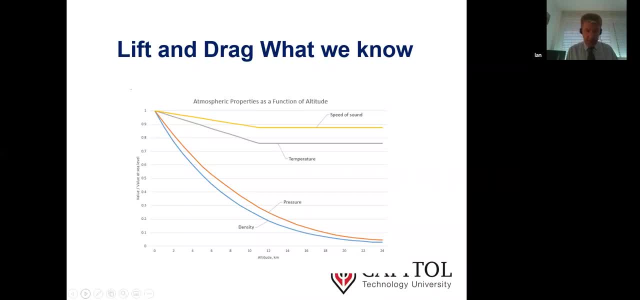 drops and drops now a lower pressure is good because if we have a high pressure under the wing we get lift but it's difficult to get that higher pressure under the wing with the density but you can see most areas of flight here there's a difference between the pressure 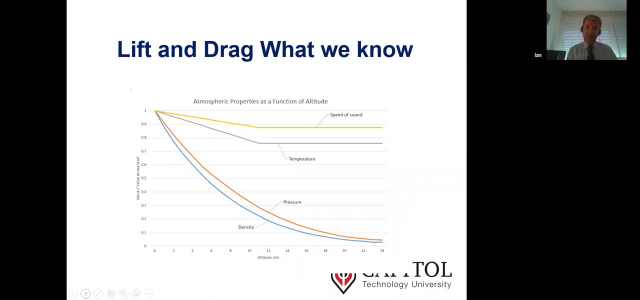 and the density and that got me thinking next slide please 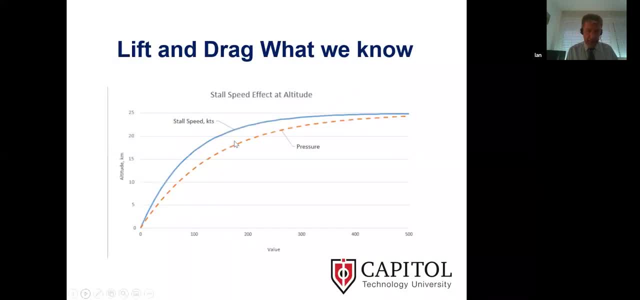 and so i re-plotted the data and was looking at stall speeds with altitude and we can see the stall speed often increases you know as we go to different altitudes and i'm thinking but there's still a difference 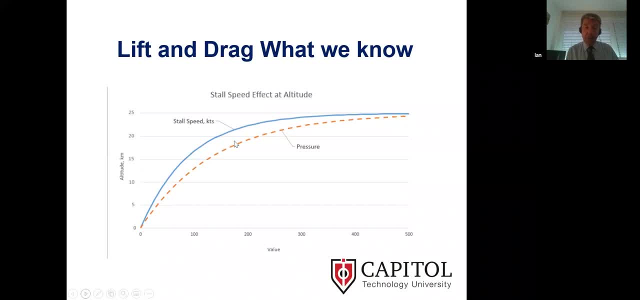 between you know what we have the pressure and the stall speed there's something there which means there's a bit of energy if there's a bit of energy we can get that energy and if we can use it we can actually start to be thinking about what we're doing now finally the next slide where i've got to we're going to really move forward in silence now 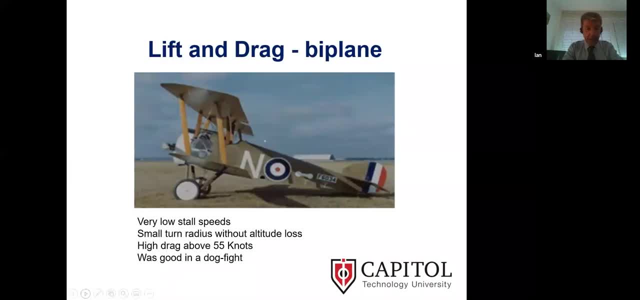 here we are this very advanced aircraft yes a 1920s 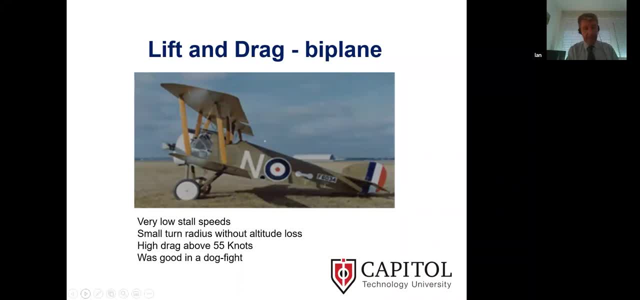 biplane you look at this and think you know this is 100 years old this thing what we're looking at this for well what i know about biplanes and if i think about sir george cayley who was investigating 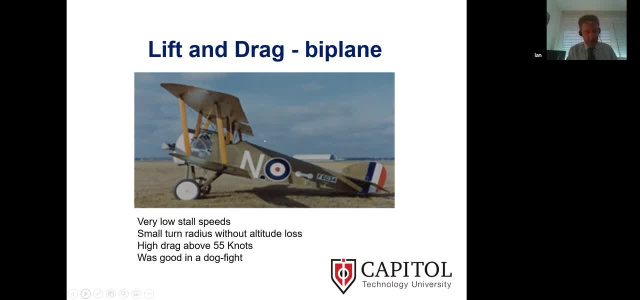 lift and drag and different things in the early 1800s and we were looking at these things here 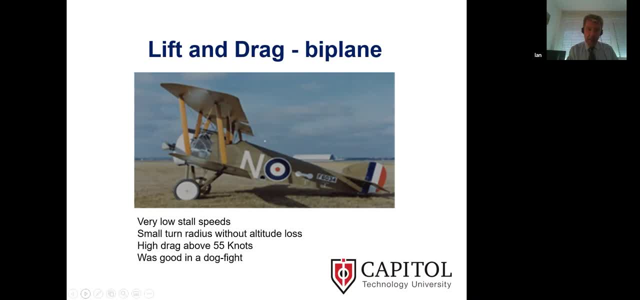 now biplanes they may be antiquated they may be laughing at but let's think about aerodynamics of them they have incredibly low stall speeds they often stall at speeds lower than most aircraft even like private aircraft take off at it's not uncommon for them to be as low as 45 knots that type of thing now that's an advantage 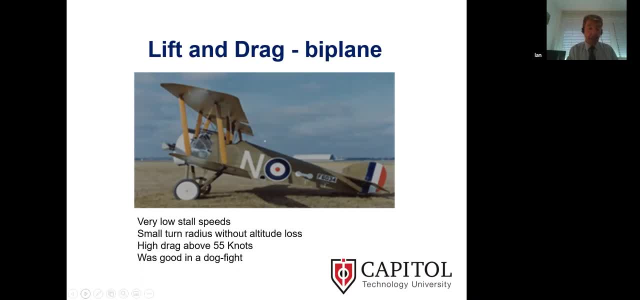 that it has almost no other aircraft it has incredibly small turn radiuses the dogfights that would happen in the first world war you know they will be turning around on a very small circle really really turning around low speed so they didn't have too many high G's turn around and you could turn around on a corkscrew type of thing and it was one of their advantages or is one of the things that made them how they worked in the war but it has an 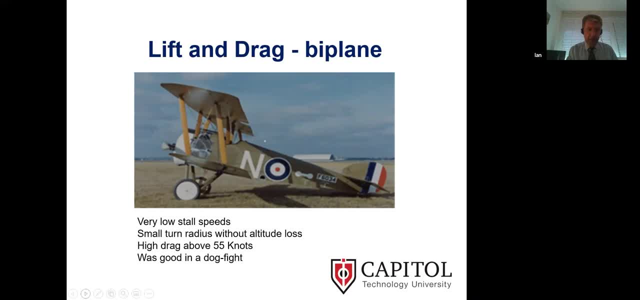 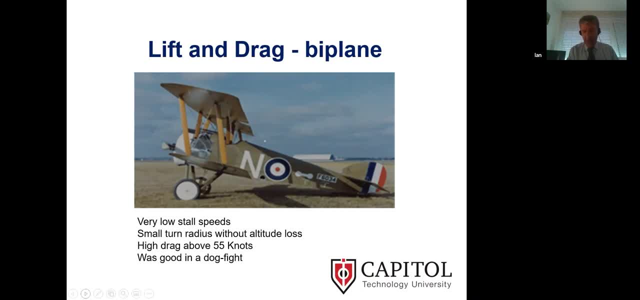 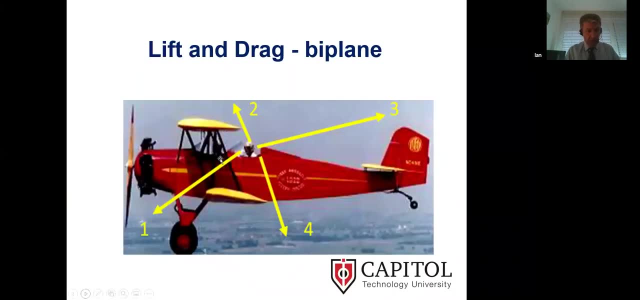 stall these are advantages but the drag is enormous the next slide please and I'm still confused here I'm thinking about it and there are four classic 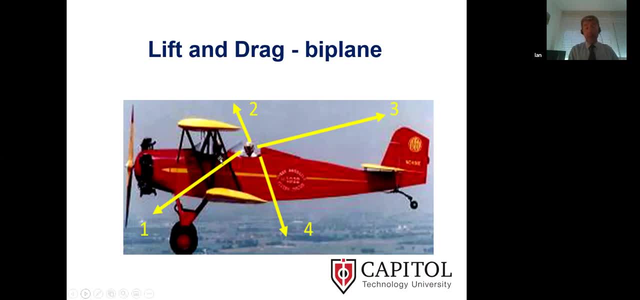 reasons of that actual or what I thought when I was just back on the map the first one being that I was just looking at the 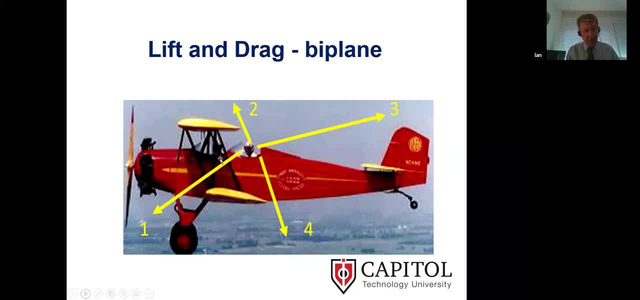 you know the I would say that that type of win computer configuration only gives you you know maybe 110 percent lift of one wing it should be giving you 200 and i'm thinking you know why is this stagger here and i could not find any research to justify 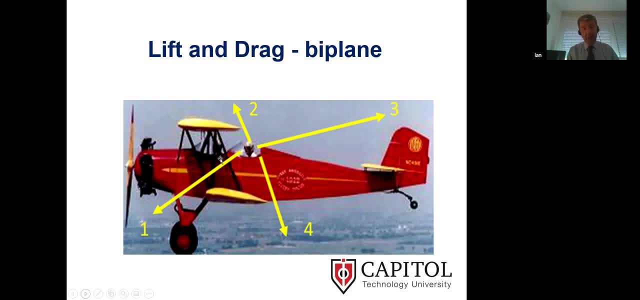 that stagger now i used to work with this man who's a retired u.s air force colonel who was also certified to fly such a biplane and i was talking to him about it and mentioned it and he said the only reason that they have that forward stagger on the top plane was really so the person could 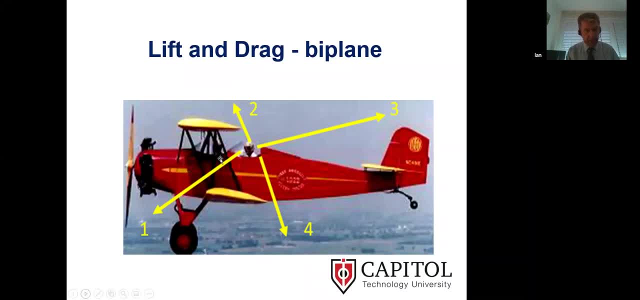 get in and out and especially when they started giving them parachutes which made me starting to think what happens if we change this configuration and this particular diagram here you can see that the struts and how much of a drag they will cause now if we can go on to the next slide please 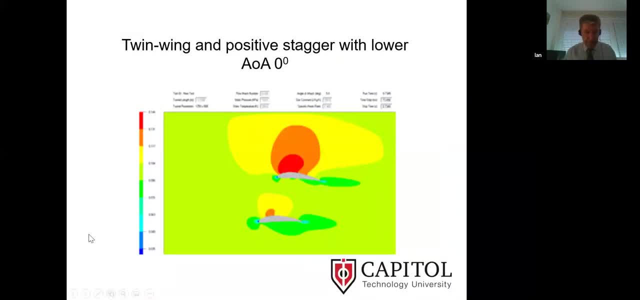 here we get and i started to do some computational fluid 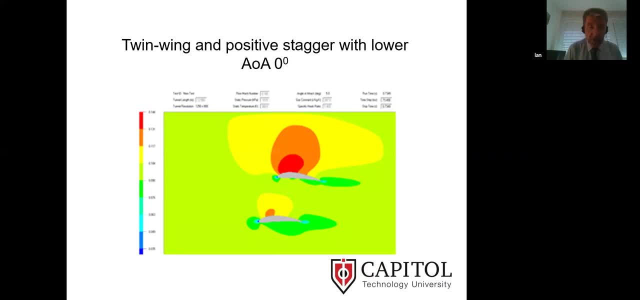 dynamics if you call it and what i'm showing here is the two-dimensional fluid dynamics that happens and i have a twin wing and with a positive stagger and you can see the top wing is behind the bottom wing with the lower wing has that angle of attack of zero so it's not twisted up it's in a straight line and if you look on the left hand side you can see the dark orange at the top and the deep blue at the bottom and what it's showing there is the sort of pressure that you can feel and if you had a brilliant wing you would have all of that dark orange above it and all of that very dark blue underneath it you will be squeezing out every bit of energy that's available for lift now this and i haven't shown you here with the forward stagger you know where it's even less but we can see on the top wing there's a nice lot of sort of low pressure above the wing and a reasonable pressure on it giving it a nice bit of lift if we look at the lower wing we can see that a lot of pressure underneath it that bottom wing in effect is not adding much to the lift next slide please 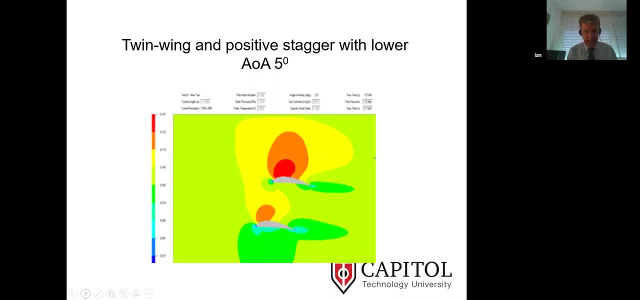 now what i did here was starting to increase the angle of attack of that lower wing and you can see that it has a little bit of an influence on the top wing but it's starting to generate more lift than the previous one with an angle of attack of about five degrees and i started increasing this again and the next slide please 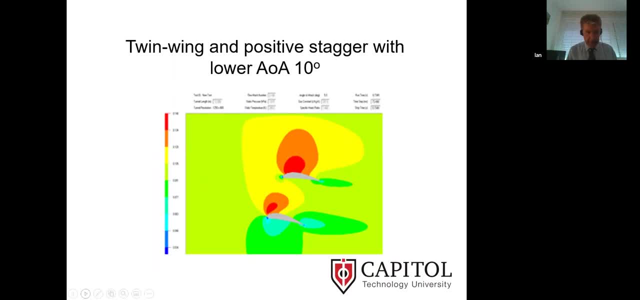 now here i've increased the angle of attack by 10 degrees and you can start to see now although it's on the leading edge you can start to see that there's a very low pressure with that orange showing it and the difference and the difference between this and the top wing we can see that it's actually substantially adding lift to what we're doing now we're going from the fact 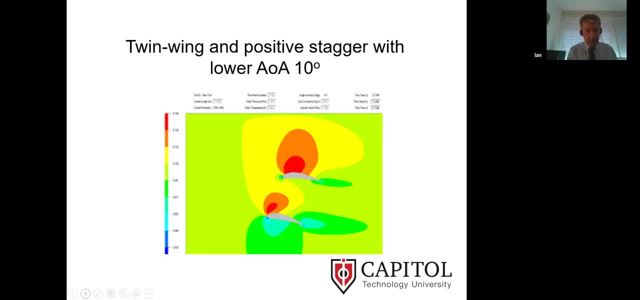 of where biplanes just give a little bit more than a single wing in its simple form 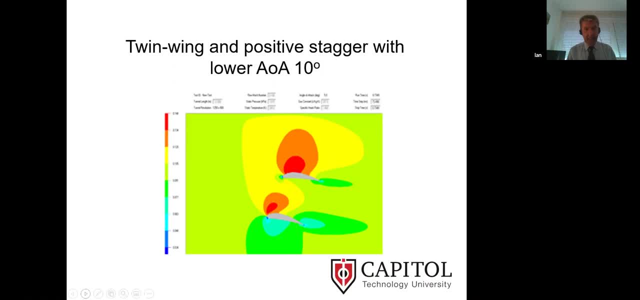 but we're starting to increase this and we're starting to increase it and anyone else that is normally an aircraft designer or wing designer or anything to do with avionics uh aerodynamics will be looking at this yes but this is no good because look you look at the angle of attack you know the drag is going to be huge on this but if we're looking to do low speeds and like a biplane configuration 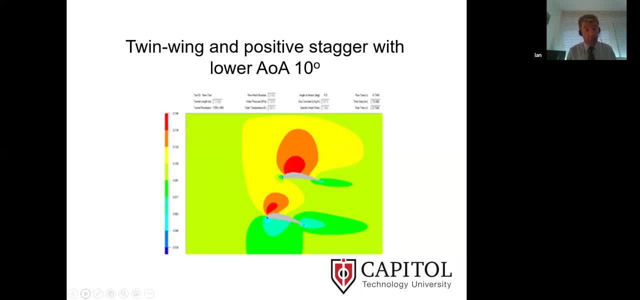 and we're flying low that drag is not so important so my next one was to actually increase it again and if you can see it now next slide please 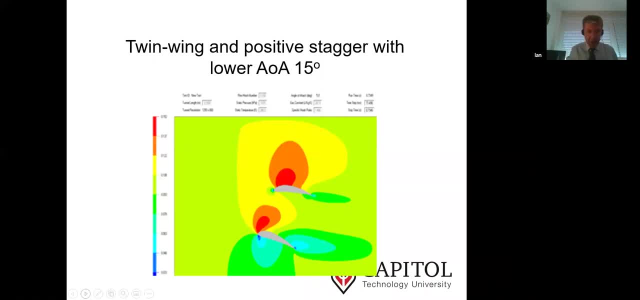 now we're here we're getting substantially a substantial increase in the lower wing this lower wing is now perhaps contributing 30 percent 35 percent maybe in this configuration there is a drag but then again it's a low speed and we're starting to see the difference now what 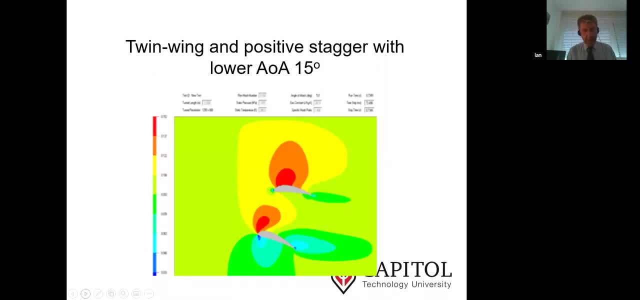 i didn't want to do today and you know i could share if you're if you're as mad as me is going 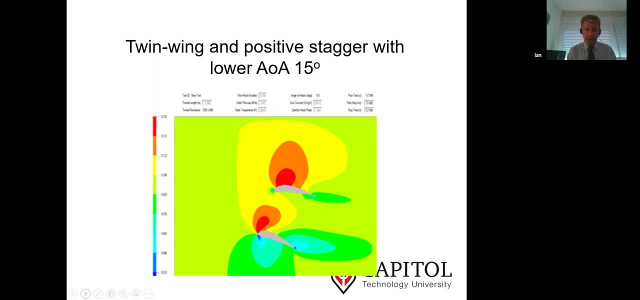 through and i believe on a two-dimensional what we call navier-stokes equation of aerodynamics i believe it's impossible i believe it is possible that we can show mathematically that in theory with the right set of combination and the right balance that we can generate almost 200 lift what you would get from one wing in other words each of the wings potentially can add the same amount of lift and that means the lower one can contribute as much as the upper one now there are lots of these and i'm not going to go through many many more of these because there's only so many you can look at without the sort of time to look at them and we can look at all these variations but it's one of the things and it's important is the airflow over these things but if we just look at this one this stagger a positive stagger with an angle of attack of 15 degrees on the lower we can see we can increase it there is a limit of how much you increase that but that's something to do another research program i have been looking by using taguchi analysis and that is where you model things as a black box with inputs and outputs and i have been doing some research and it's been published in several different sources where we're looking for the optimum height 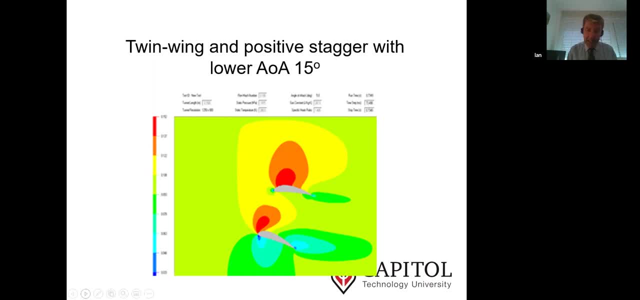 between the upper and the lower wing and the optimum stagger the offset and the optimum combinations of these angle of attack and I'll talk about that in my 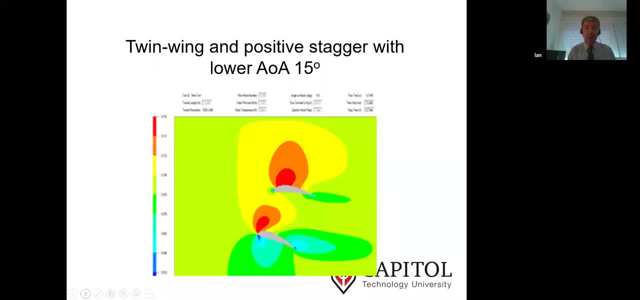 conclusion but the next slide is a slight variation in the results of the 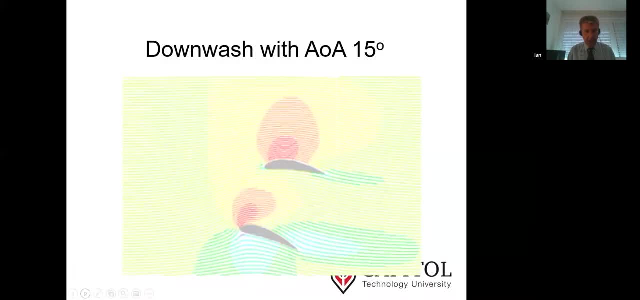 airflow and if you can do that please now this is what we call the downwash now the downwash is what is the flow and I know it's a little bit faint but I hope it's clear enough on your screen you can see that the laminar air flowing in as it starts to go over each of the wings we can see the laminar flow it's important if it leaves laminar flow to become turbulent then we have a problem lift doesn't exist and this is another problem with aerodynamics and we can see that the downwash with these limitations and we can check the downwash with these limitations and that is very important because one at the 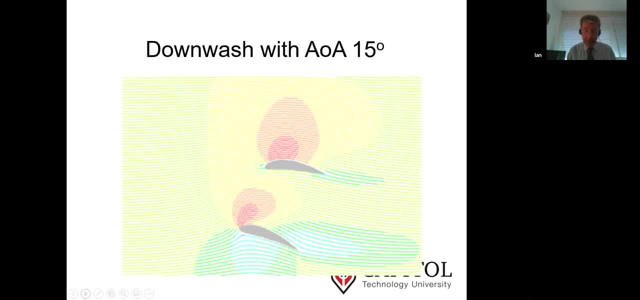 back of the plane we're normally going to have the horizontal stabilizer if that is not sorted out properly you know we cannot control the pitch of the plane because the air is flowing in very strange ways to cause problems so check in these things and what I put here today and what I've tried to do is just put a summary of 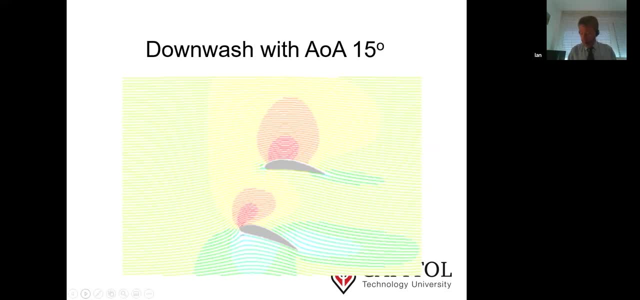 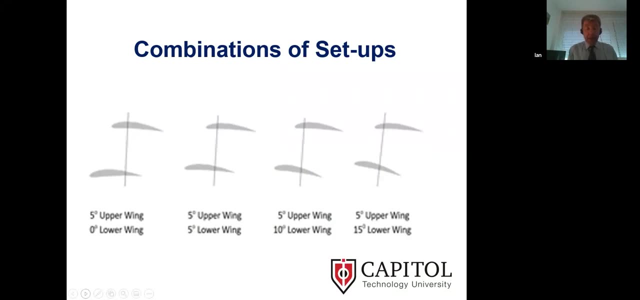 these things and if we look on the next slide please Bill and this is what some parallel research has been looking at different combinations of angle of attack on the bottom this is what some parallel research has been looking at different combinations of angle of attack on the bottom the 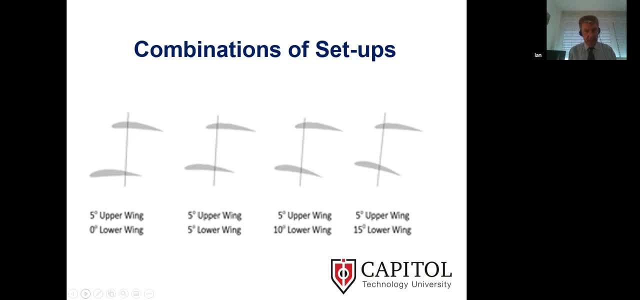 offsets and this only shows the height and there are combinations and these are subject to more sort of research and even three-dimensional modeling because I've ignored the influence of the fuselage how that if we actually look at these and bear in mind with now modern composites and different things like this we don't have to have the support between the wings we can use wings and if you think of how a glider works you know it has long wings with no support on it and if we look at these prints of wood modern materials it is possible that we may even be able to control the height between them the stagger and certainly the angle of attack of each of these wings during the various stages of right that are necessary and of course that is to be able to take off first of all and then to be able to climb to a very high altitude and then remain at 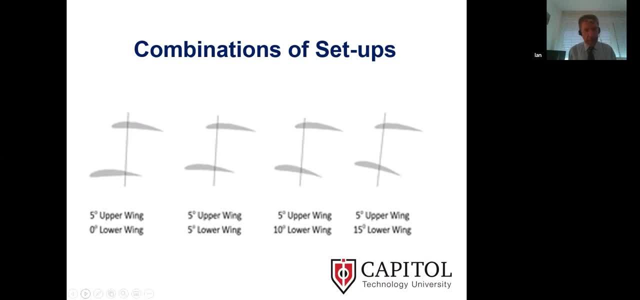 that altitude with a relatively low forward speed to give us that we could potentially use UAVs to control the height of each of these wings under the levels of envoy seasoning and radar vehicle 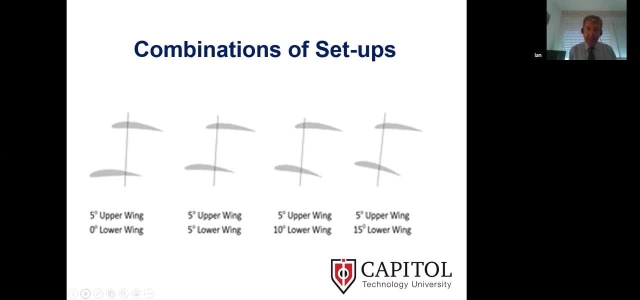 to fly at high altitude. If we do not need speed, 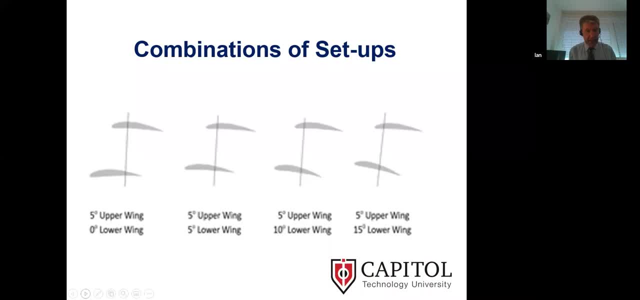 we drastically reduce the engine power needed. That means we drastically reduce the weight of that engine propulsion system. And this is where it fits in with UAVs. 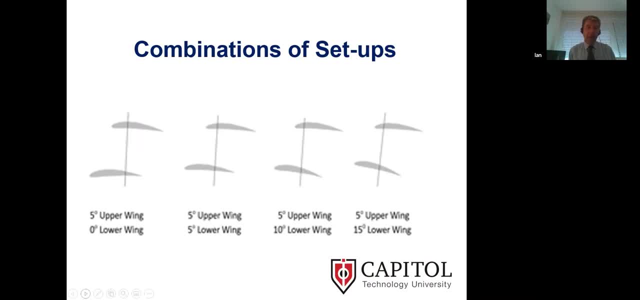 And my research, and I'm doing this as sort of, it's been a thing that I've been doing for a couple of years now, is coming up with this and looking at this. And one of the key things is the propellers. Because propellers, if there's very little density at 40,000 feet, again, you need to squeeze out the maximum energy from that propeller. 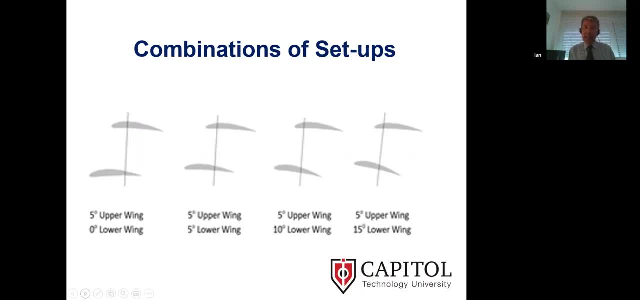 And if I go back and we talk about these things, and I mentioned the DC-7 at one stage, if you can remember several slides back, that was one of the first successful commercial aircraft that used variable pitch propeller to alter in takeoff, in altitude, in approach, reverse thrust in landing. 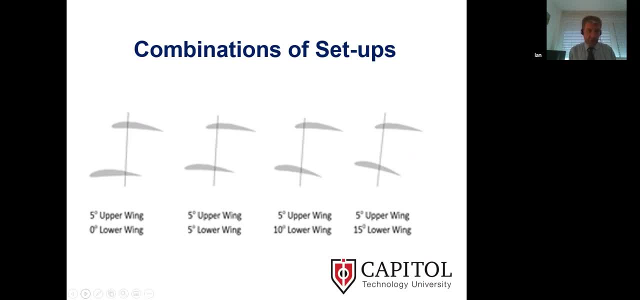 If we move this forward, and we look at some of the modern turboprops, and if we look at some of the blades that are on the C-130s now, for example, or the M-400 from British BAE Systems, sorry, Airbus, if we look at those, they're even more, they're sabre shaped. They squeeze out every bit. And this research is going on parallel with my research that I'm looking at on the propellers. 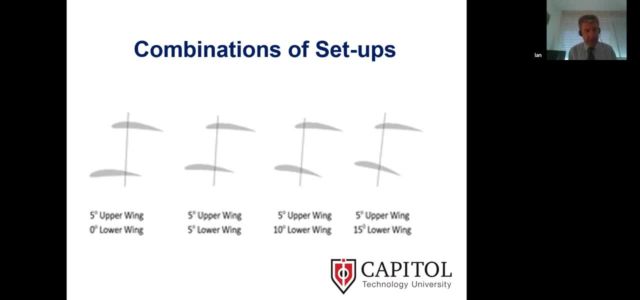 And I'm still trying to show in three-dimensional Navier-Stokes, I'm still trying to show in three-dimensional Navier-Stokes, how we can match this and work out the optimum from it. 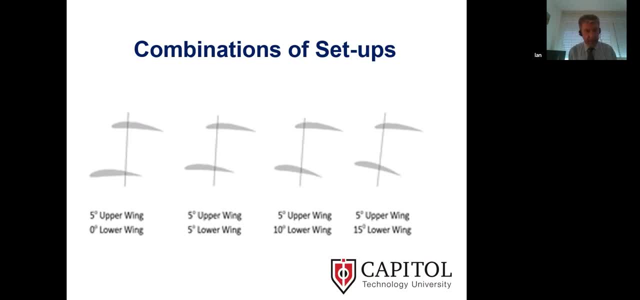 Now, there are some aircraft around now that use this type of stagger, but they tend to be a very low distance between the bottom and the above one. And that has its implications because of minimising drag. 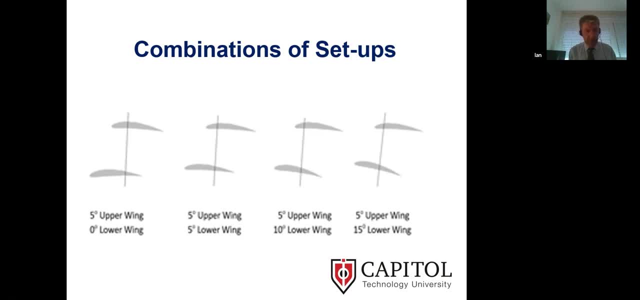 But most of them don't look at this massive alteration of the upper and lower wing angle of attack. Research has not bothered about the speed at low speeds for years, because planes could go very, very fast on the ground. 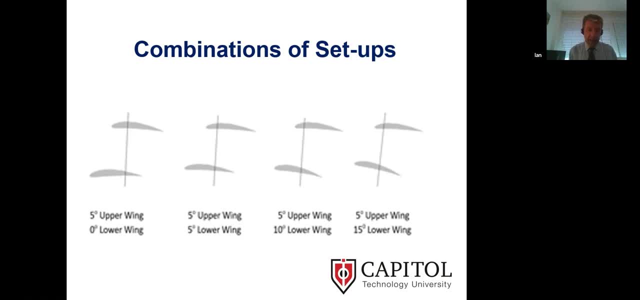 We don't want drag, so we don't look at the angle of attack on data. And we ignore that with all our new designs. 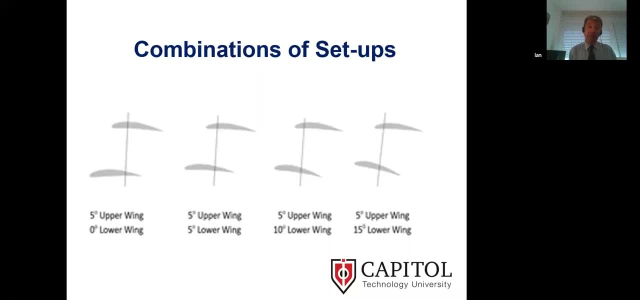 And I think in some ways, when we're looking at this, we need to be thinking about, and going back to my Jurassic Park quote, don't ask, should we do it? We could ask, you know, should we be doing it? And at the moment, we haven't got the answer 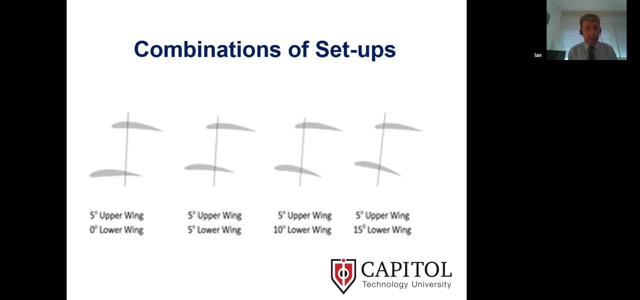 about using UAVs in commercial or where it can fit in. 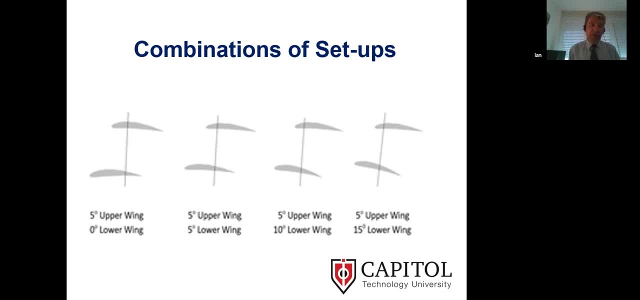 And I think by actually looking at this, and if this research is successful, and it does culminate with being able to prove things 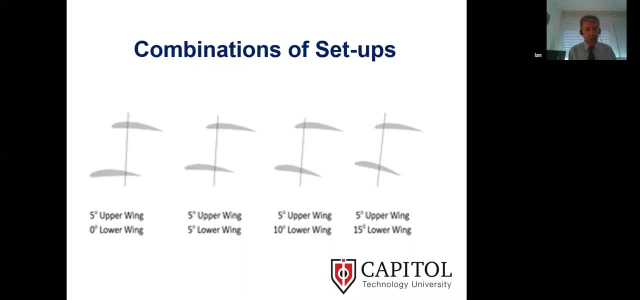 before we make prototypes and try to fly them, it totally separates the actual commercial and potential UAV for long distance. 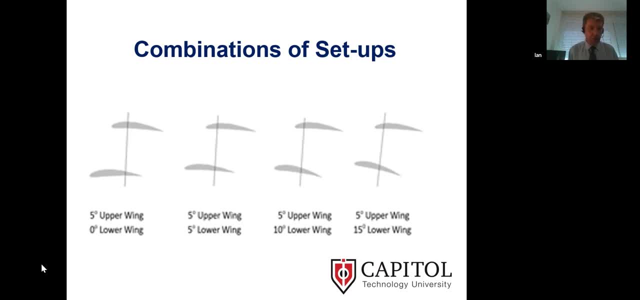 Okay, you fly up to an altitude in commercial space, but that's easy, just the same as a military airfield. You put like a cylinder in that area and you can corkscrew all the way up and different things and keep away from everything else. Next slide, please. 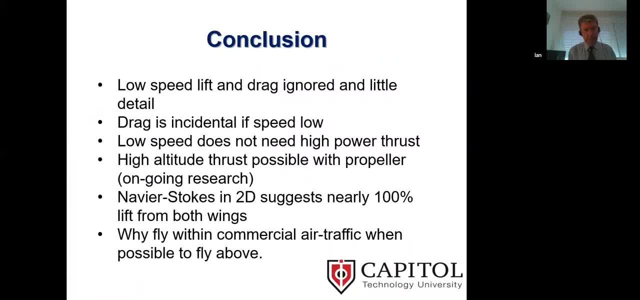 So my conclusions, and what I'm trying to say here today is that low-speed lift and drag ignore in little detail. People haven't looked at them for years and have totally ignored it. Think about your own area, whatever that is, you know, whether it's manufacturing, cybersecurity, data analysis, people ignore things that were done in the past. 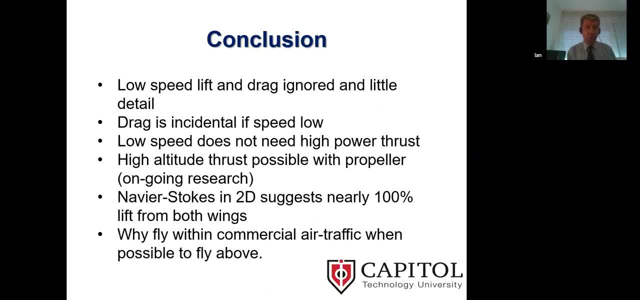 Ah, I don't need to do that. You know, it's not relevant. It's not useful, different things like this. 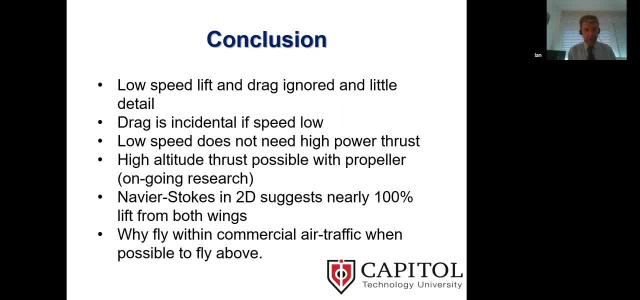 Look at a really, weird sort of comparison with uh let's say cyber security you know carrier pigeons what a brilliant 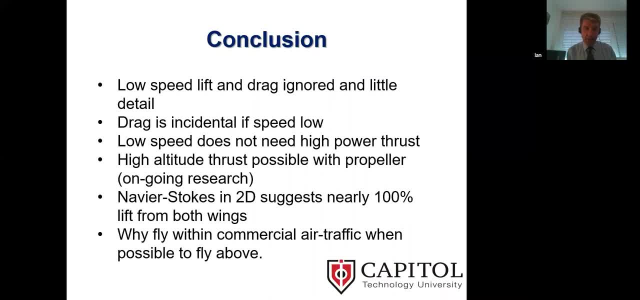 way of getting private information from a war zone back to the headquarters doesn't matter how big your quantum computer is you can't get that carrier pigeon you've got to shoot it down and mechanically get it there are solutions from the past which may be useful for today and i believe 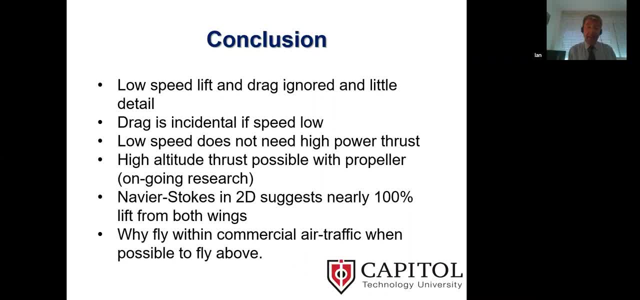 this is the so when it comes to uavs drag is incidental at low speeds it's something that's not really a problem low speed means we don't need high power you know there's a lot of design of the propeller that i'm looking at and how we're doing it and just for your own sake if you go and look at one of the pictures of an old biplane it's made out of wood with a fixed propeller you try and find a quad cop a quad uav being used now that has anything but a static fixed propeller 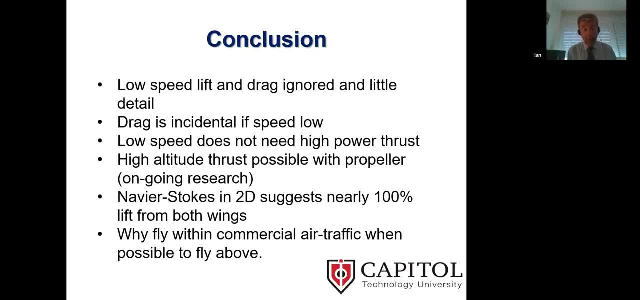 as opposed to a variable one which is used in real commercial flight now and again my navier stokes is suggesting 2d that we can almost get 200 100 lift from each 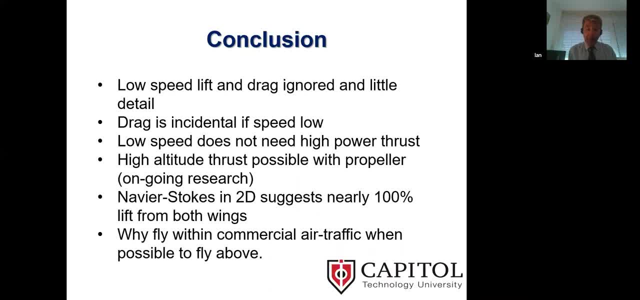 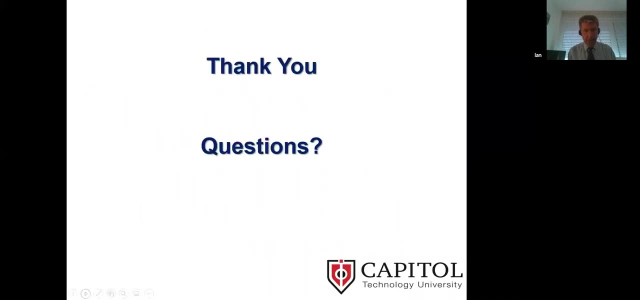 wing without affecting the other one and i would like to finish by saying why fly within commercial airspace when there's all that risk when maybe there's a possibility to fly above it so next slide please i'll say stop there thank you and questions i was told to finish at quarter two and 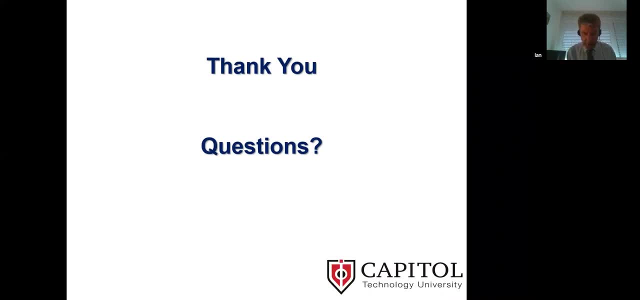 quarter two so if anyone if you can let me know some of the questions if there are any in the chat box it's too small on my screen to read but if there are and i'll try to look at it i'll try to answer any questions if people have okay let me jump in here thank you ian um there are a lot of 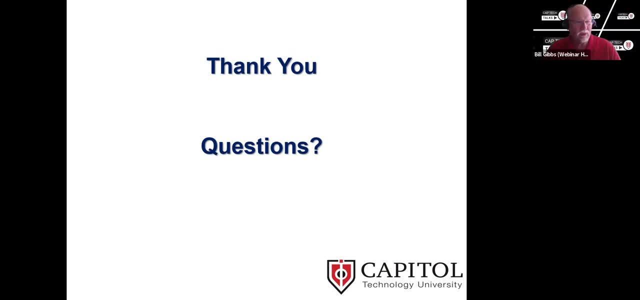 comments they're not necessarily directly related to your last part of your presentation they have a lot to do with supersonic flight philip mentions that an arion as2 is a 12-seat supersonic private jet hopefully we'll be ready by 2026 there's still couldn't couldn't agree with him more you know it is fabulous and i really really hope that happens and yes they're pushing forward noise might be a problem for certification but let's hope it happens all right laurie uh says do you think commercial flight and the and space flight will meet somewhere in the middle in the near future where prices are not so ridiculous such as spacex and allow commercial flights to reach above 60 000 feet again i absolutely think they will do and it's got to be done you know if you look at the virgin galactica and also there's the other founder of 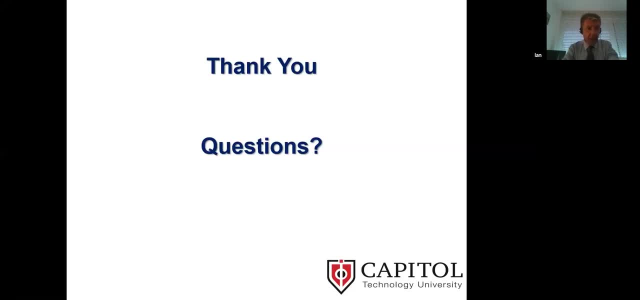 microsoft wasn't he was looking at those things i don't think we're too far away and you know you really need to be doing 70 to 80 000 to see the curvature of the earth and then throw away your membership for the flat earth society but i think it's got to happen you mean there's no flat earth 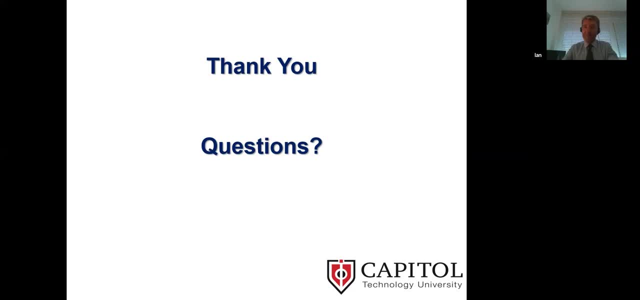 i haven't been at 70 000 feet i couldn't possibly comment all right uh soren has a very interesting series of two chats that he talks about a supersonic airliner called overture and that is designed to fly at mach 2.2 and has a price tag of 200 million dollars but it's they've got pre-orders already from a number of different major airlines and they hope that they can make supersonic flight would be available from new york to london for 2 500 um that would be wonderful 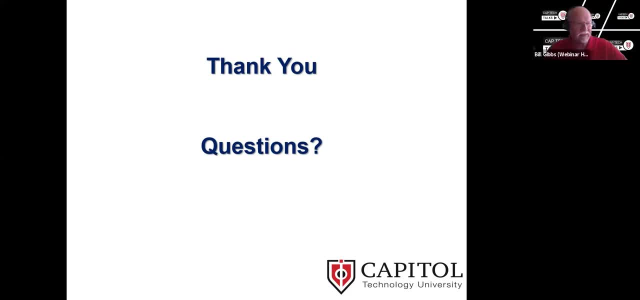 how long that would take but it would not take very long i can tell you i can remember my father years ago in the sort of late 70s he used to do day trips from london to new york day trips he'd 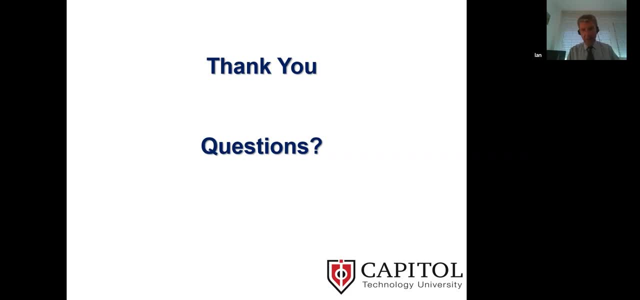 get the six o'clock flight out of seven o'clock out of heathborough and he'd land in new york at sort of five o'clock in the morning and be in new york city at seven o'clock do a full day's work there he'd wrap up at seven o'clock and he would be on time for a full day's work he'd be on time for another five days he'd be on time for another six days he'd be on time for another five days um he would be on time for another five days he'd be on time for another five days and he worked 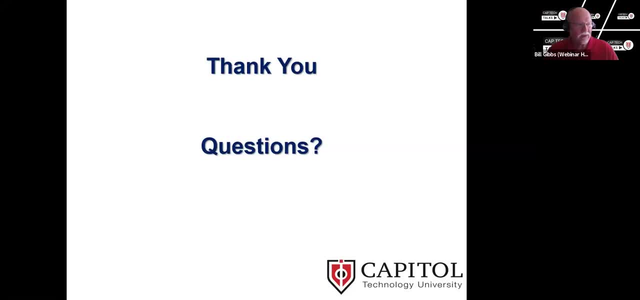 three days in a row with small fog lights on the cie которые he'd be in charge of that was a long time and i was back in london for the first and last forest season and it was super excellent i remember being in the for the first and last forest season i got to see this the next year and i was working hard with it and it got little by little and the brothers and daughters were normally free but in london and every year before the schools were open in the spring it was And if you can amplify that remark, I'd appreciate it. 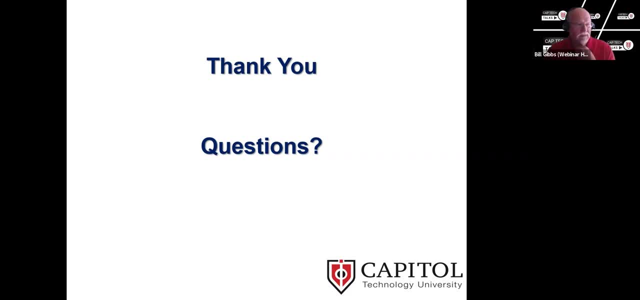 Marvoy asks, several drones flying in proximity at varying AO. Angle of attack, yeah. Okay, so could you maybe amplify how that might work? Well, I mean, worst case scenario, UAVs flying, is that they hit each other and there's a crash. 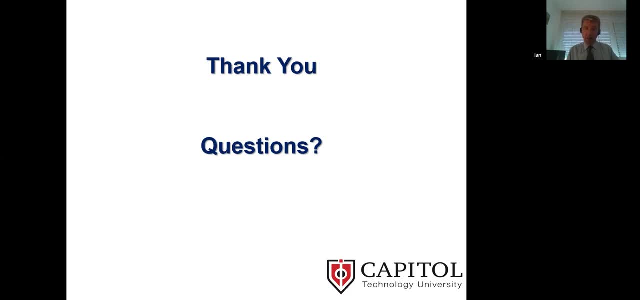 And the possibility of that damage then hitting a commercial plane below and then landing because it's so small, it is much different than two commercial planes hitting. But we have TCAS, you know, that tracking to avoid system. 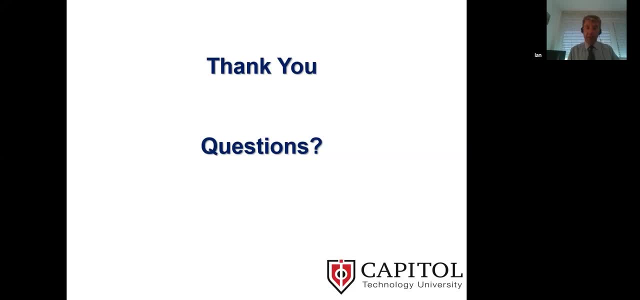 If you ever go on gliding, if you like aerodynamics, you've got to go gliding because it's really aerodynamics. 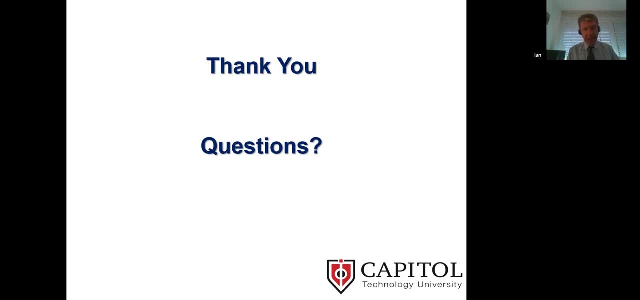 You know, there are low cost machines or devices that gliders have that cost a couple of hundred dollars that you can install to prevent actual collisions and different things like that. And I know there are military planes that fly at high altitude, but they have jet engines. 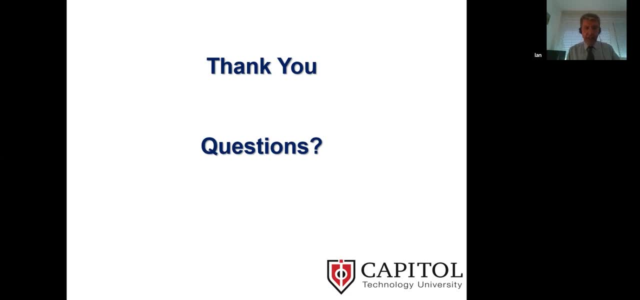 They have a lot of information on them. They're not really designed to carry a payload. 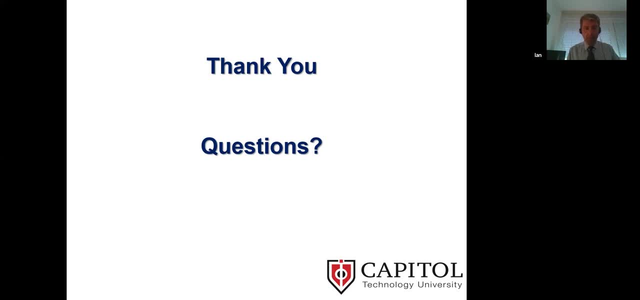 And I'm looking at the fact, and in some ways, I'm ignoring the commerce of this particular type of research. I'm looking at it as, can you have a low speed, high altitude, low cost technology product that can fly above that area? And now it may never be commercially available, but it might be. 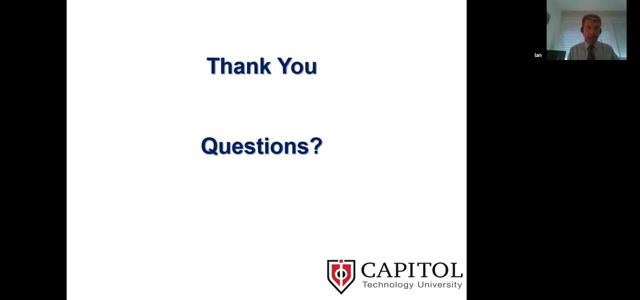 And if you could do that, you think, you could put something on a plane and you could fly it across the Atlantic. And you don't care how long it takes, if it's something to be flown across, because if it takes, it flies that whole 24 hours and you're sending something. Well, just imagine what you could do if this was in a disaster zone, 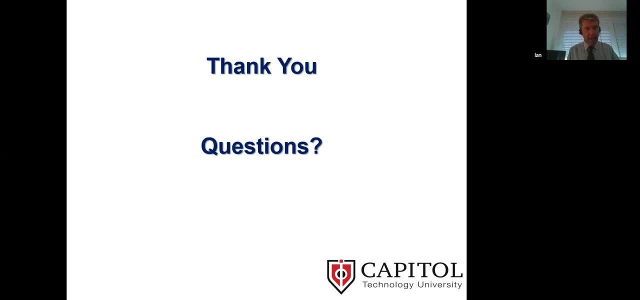 where you think of that horrible, what happened in Haiti a couple of years ago, you could fly this at 40,000 feet with a little bit of information in there to get the mobile phone system working again with a transmitter on it. 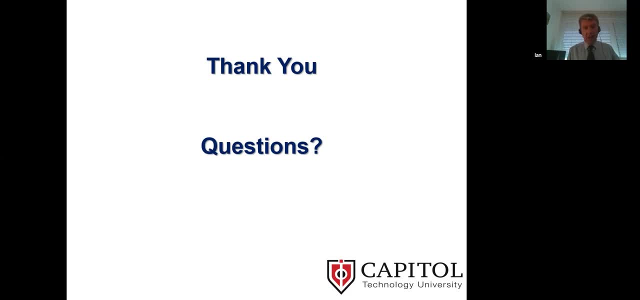 And some of those applications or, you know, you're searching around for something in the sea, you know, low cost drones and we could fly them around. And if you're talking, as you were with your bigger question, imagine if we have quantum computers controlling all these drones, you could use them as forms for looking at things. We're looking for lost people for monitoring the sea or anything else like that. But that's probably beyond what I'm one interested in too, is looking at, I just want to solve the propeller and then make a prototype to try and get in high altitude at very low speed. And I think maybe under 60, 70 knots, theoretically, I believe is possible. That's interesting. And you mentioned just now quantum computing. 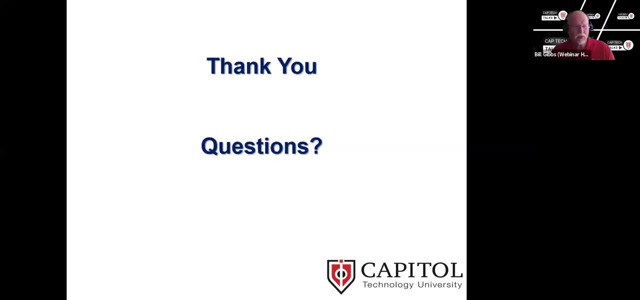 Cindy had asked the question, how can, how do, how drones be controlled when they're that high? 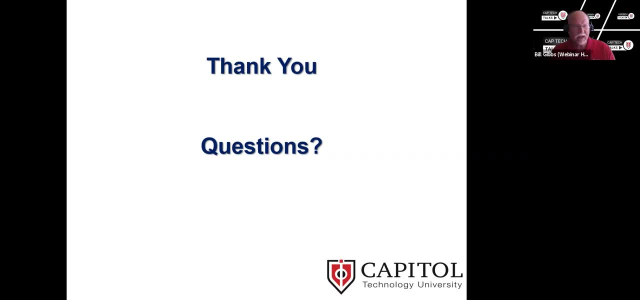 And, you know, obviously they're not line of sight. Well, they certainly be on line of sight. 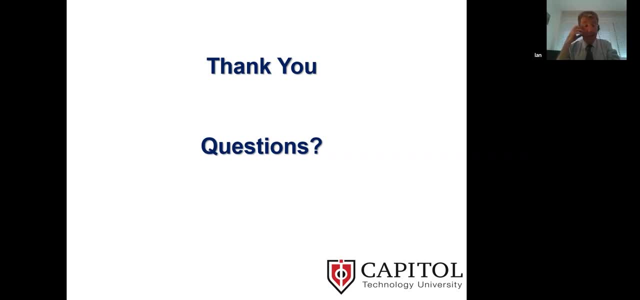 But if we look at quantum computing, we're also going to have some form of artificial intelligence. And therefore, the up to surface to air communication isn't necessarily going to be that critical because artificial intelligence should be, once we have the quantum computing working commercially and available, the AI should be a step ahead of that. 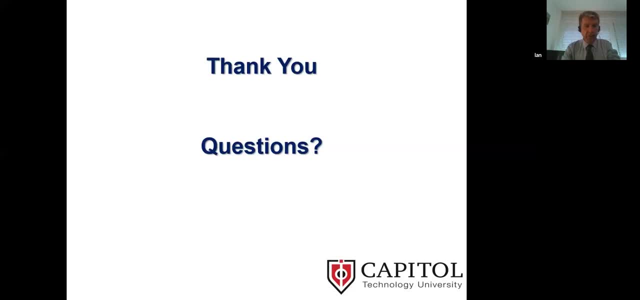 And I would see that the AI is probably doing that and whether that's military defense or any other things. 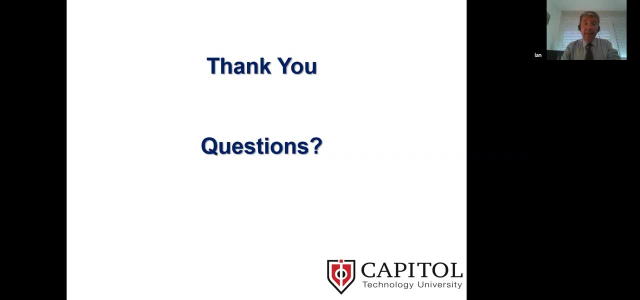 And, you know, I don't think that will be a problem. You could even do it from satellites above, couldn't you? Low off the satellites. Yes, that's true. 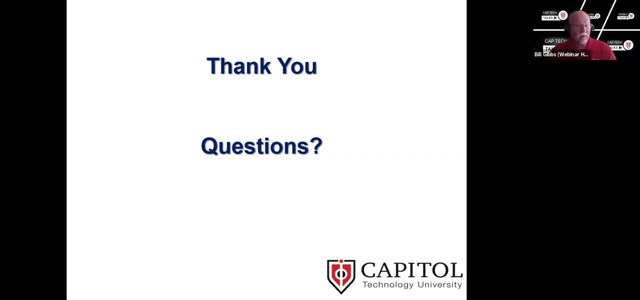 The, taking a departure from the questions that were directly related, you mentioned the 737 MAX and Lyndon asks, what's your take on the risks and problems with it? And again, this is a little bit of an offshoot from your actual discussion. Not a problem. 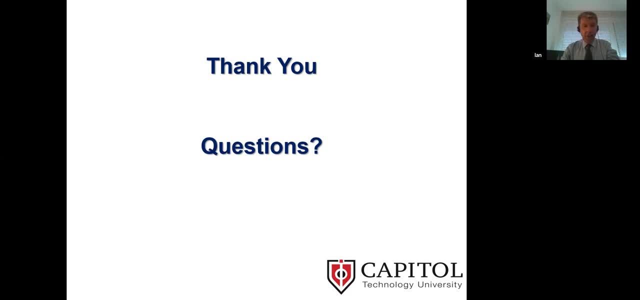 I mean, if we look at it, you know, there's two ways you can look at it. One, the 737 is a brilliant plane. But like with anything. I think when you keep stretching it and modifying it and increase it, you get to a point where, you know, you don't get the same as if you start from the beginning. And they've been trying to make that as it's a backbone of aviation across the world and balancing those things. And they got it all right. 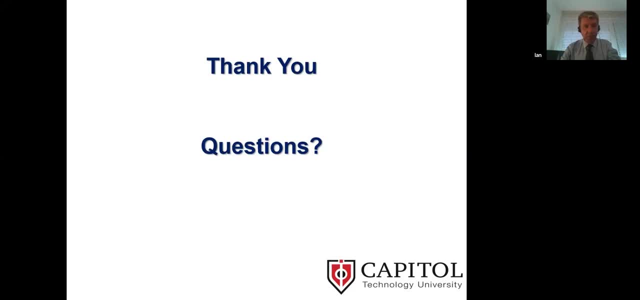 The only thing they really got wrong was a little bit of the software, programming the software, the warning systems of the pilot, and they've lost confidence in people. And that's the problem, is the confidence. If we test all systems. 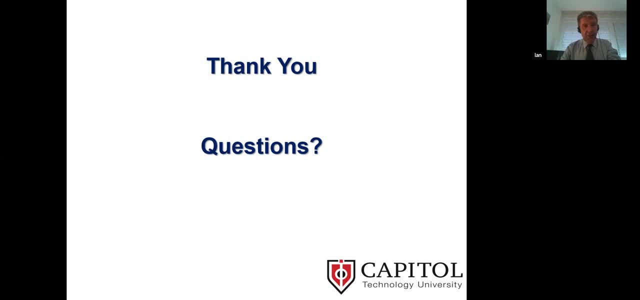 If we test the software, there's always a bug and I have to say, I hope that the 737 MAX is flying soon. I believe I was, someone told me, you know, there's something like about 800 waiting to be delivered and they haven't got enough pilots to deliver them if they were instantly told that they could do it tomorrow. 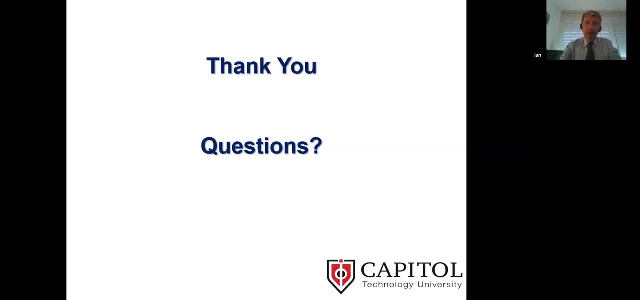 You know, it's important. And, you know, and I think, and sort of, if we go back and until Airbus really challenged, you know, the commercial Boeing were a little bit lazy in terms of upgrading. But I think it's the same thing. 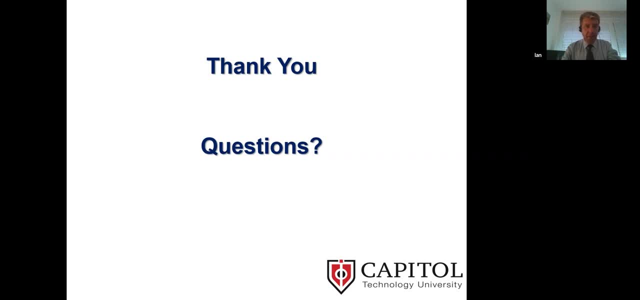 I think the whole point of the 737 MAX is to have a lot of efficiency in flight entertainment. Competition is good and we, as customers benefit. And I hope that the 737 is approved to fly again soon. 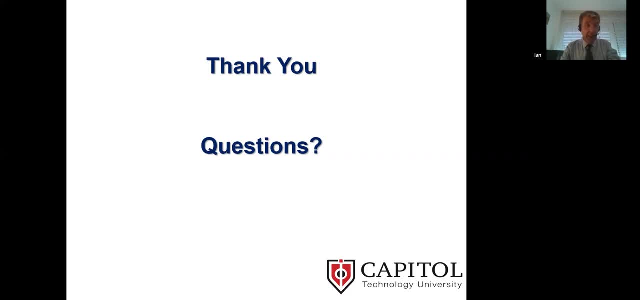 It's as a technical problem, it's not huge. I think it's a political and economic problem. It's something beyond my intellect. I would say. I see our time is getting away from us. 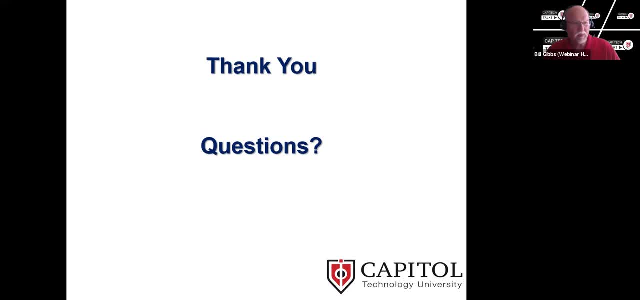 And so I deeply respect our participants and audience members time. We will end at the top of the hour, which means, unfortunately, that not every question will be answered. 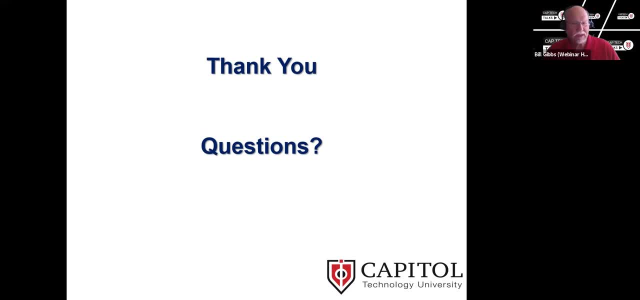 I will save these questions and forward them to Dr. McAndrew, and we may have to have a second session just to deal with some of these questions down the line. 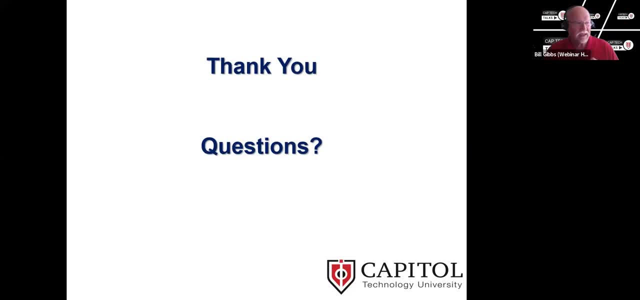 I'm going to ask one more question because this one actually deals with your question. 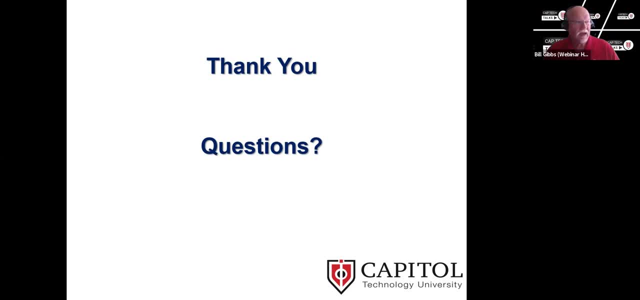 SG Stanford says, looking at the last slide of the bottom wing angle of attack, it displayed the low pressure on top side interfering with the top wing's leading edge high pressure region. 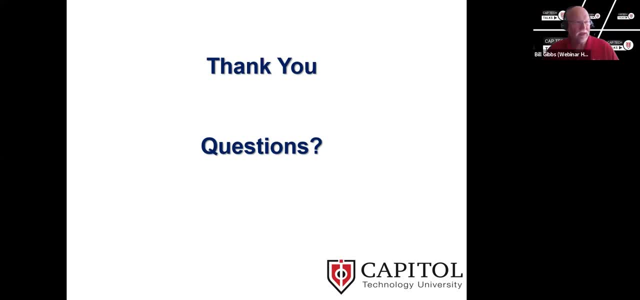 Can adjustable slats on the upper wing help divert the interference from the bottom wing's high AOA? Absolutely. I don't see that as a problem at all. 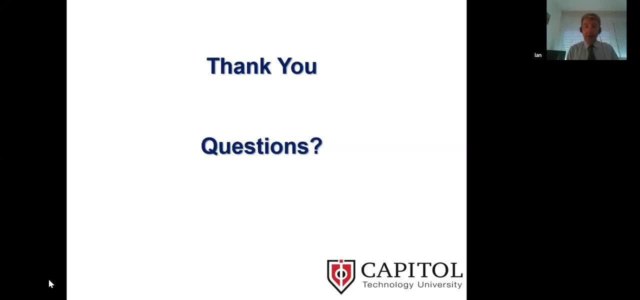 The only technical problem really is that if you have a wing that requires the slats, then you're starting to add complexity, cost, and weight. 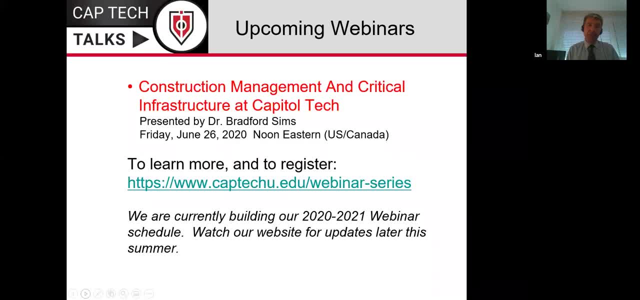 If it can be avoided by looking at optimums, and if you're interested, if you look at some of the actual... 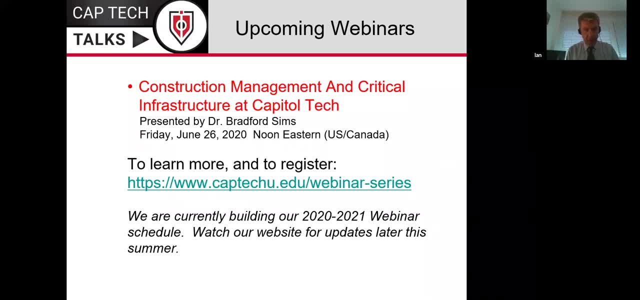 If you Google some of my presentations, you can see some of the research where I'm talking about that, and I'm delighted if you look at it, and if you've got any questions, even more delighted if you wanted to get into a conversation like this. 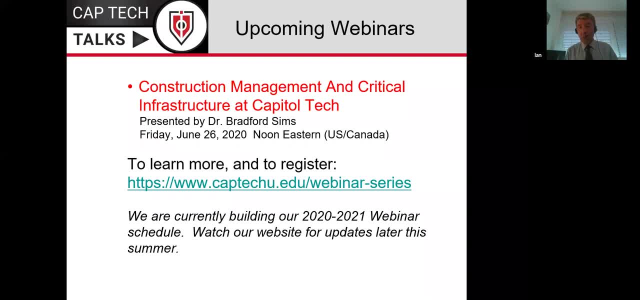 It's a sort of area where if you're sitting on a long-haul flight and you start talking to someone about this, they automatically think this is going to be a longer flight than normal, but occasionally, some people want to hear, and it's always wonderful to talk to other dilettantes, if I may say. All right. Thank you. Thank you. And again, if you had a question... And we did not get to it. 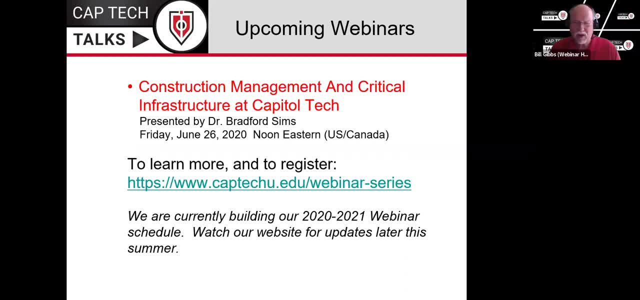 I do apologize, and we want to deeply respect all of our participants' time. I want to move on now. First, thank you, Dr. Ian McAndrew. It's been a wonderful presentation. I really have enjoyed it, and I'm sure everyone else has as well. 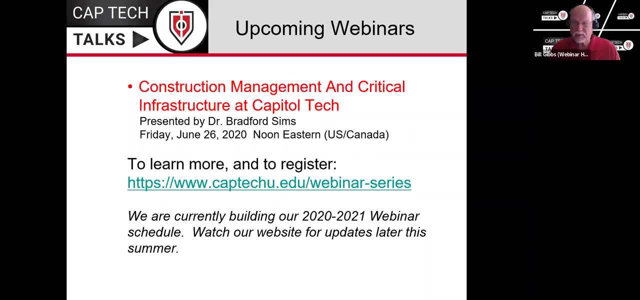 Our upcoming webinar, we have one more this spring. It's going to be on Friday, June 26th, with our president of capital, Dr. Bradford Sims, who will be speaking about construction management and critical infrastructure issues using capital tech. 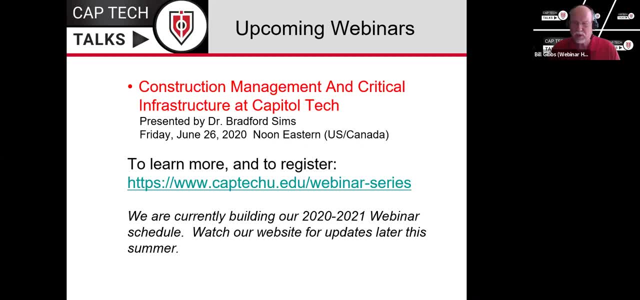 He's going to give us an example, but this is an up-and-coming area, and I'm sure you'll want to join us for that. 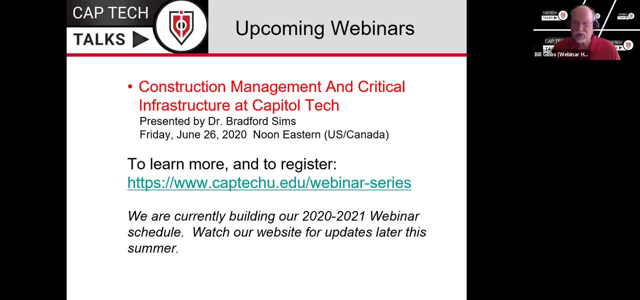 We're currently building the 2021 webinar schedule and be watching our website for updates later this summer. 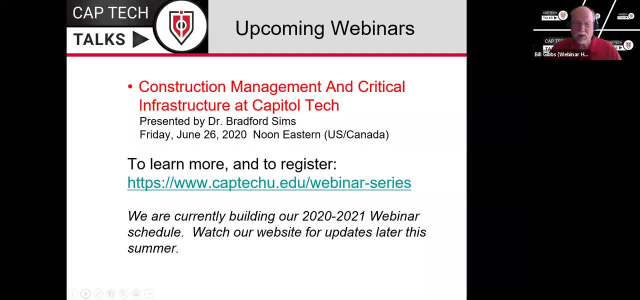 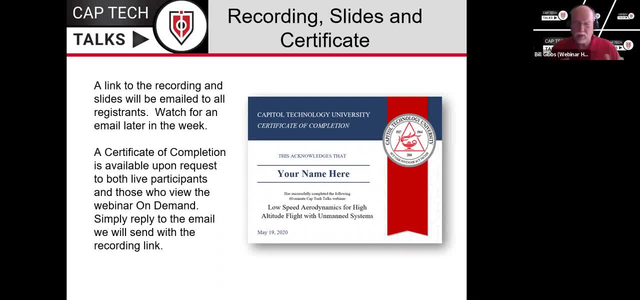 I think we'll do it. And that includes registrants who were not able to join us live, although most were, 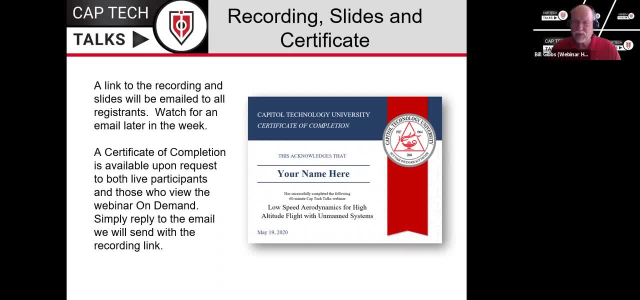 and all of those who signed up for this. Watch for that email. 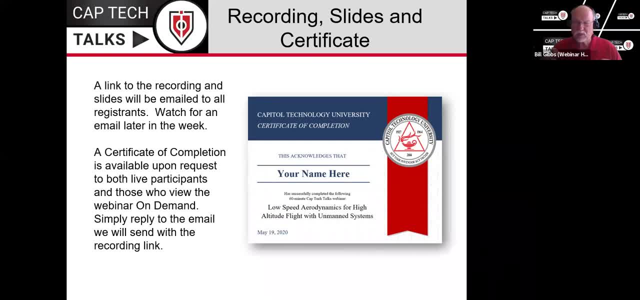 A certificate of completion is available upon request. When you get your email from me, all you need to do is reply, yes, I want one. Here's the name I want on the certificate, and I will send that to you. 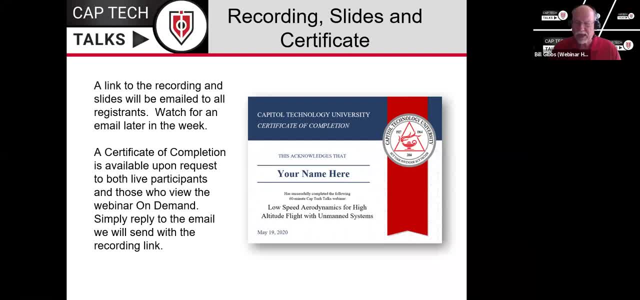 I'll do that also once you have watched it on demand for those who are listening to the recording as you hear this.